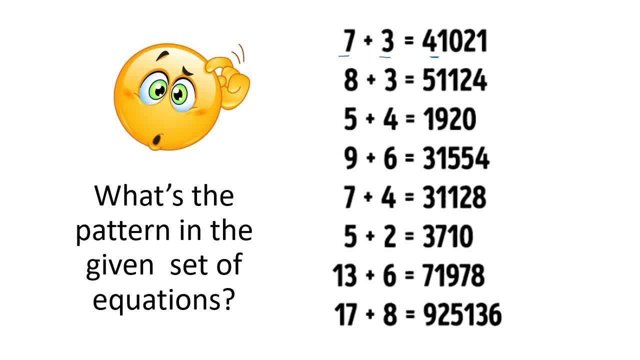 You have 7 plus 3, and then you have 4 here. So what happened? This is 7 minus 3.. Then for this one, the second number is 7 plus 3 and then, lastly, it's 7 times 3, right. 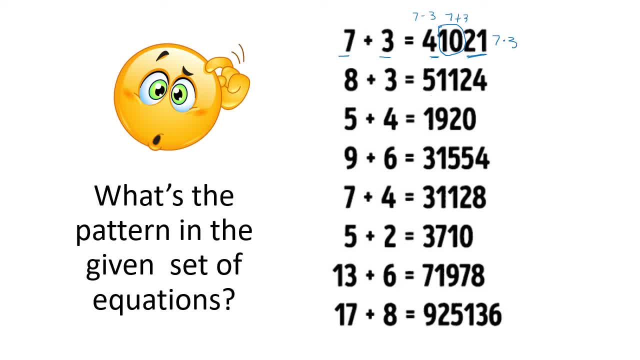 So let's see if that is the pattern for everything. So for the first one, 8 minus 3,, correct. And then 8 plus 3, and then 8 times 3, right. So you can verify that for everything here. 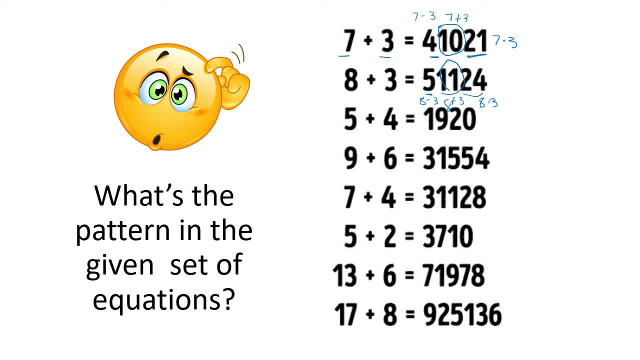 For all the numbers here. that is the pattern Let's just look at. take a look at the last one. So 17 minus 8 is 9.. 17 plus 8 is 25.. And lastly, 17 times 8,, 17 plus 8 is 25.. 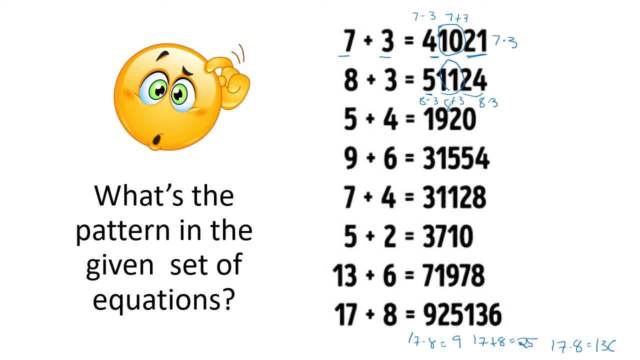 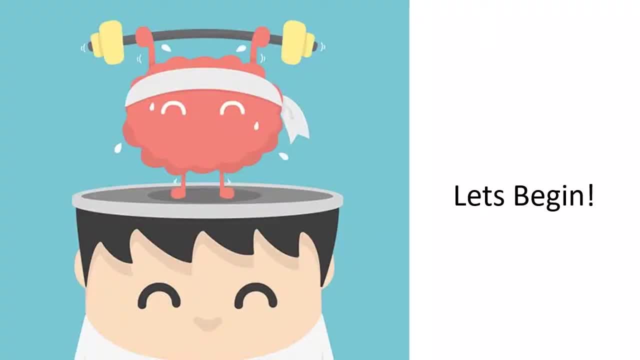 And then 17 times 8 is equal to 136.. Now that your brains are all warmed up, what I just want to show you is that many results in mathematics came about as a generalization of patterns and shapes. Studying patterns allow us to observe, hypothesize, discover and create. 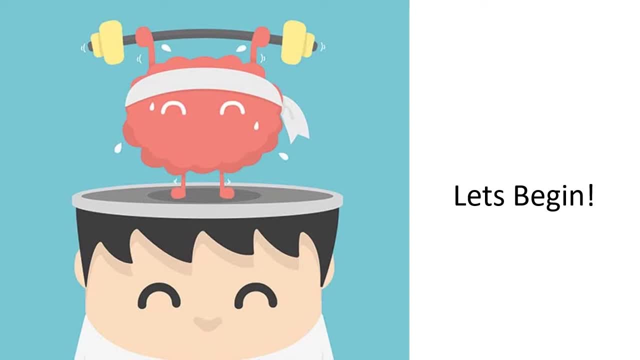 So take note that the way of doing mathematics now has evolved from just performing calculations to making deductions from patterns, testing conjectures and estimating results. So now that you're already in college, so math is just no longer like what you're doing in, probably in grade school. 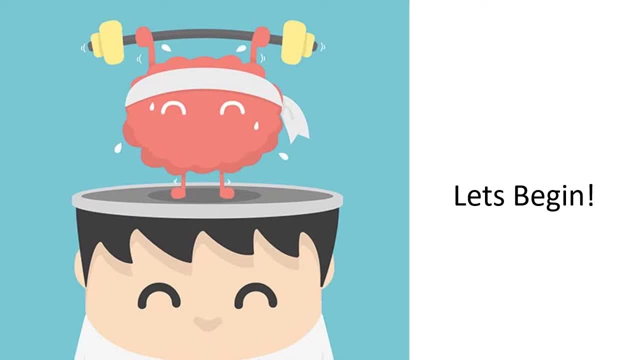 where you just have to multiply big numbers. It's just a series of calculations, right? So of course, mathematics allow us to think analytically. So all these aspects tell us that we have to in order to progress with the help of mathematics. 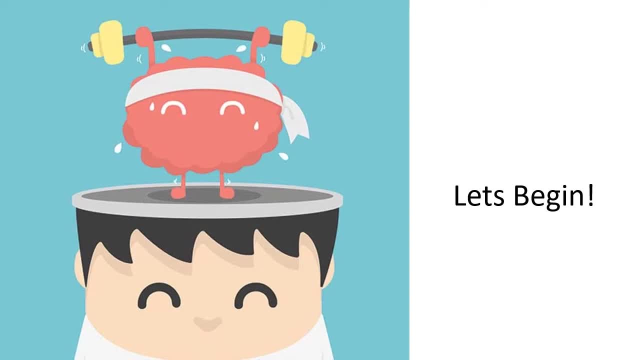 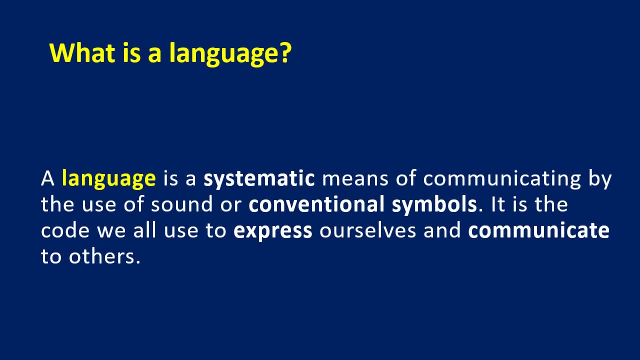 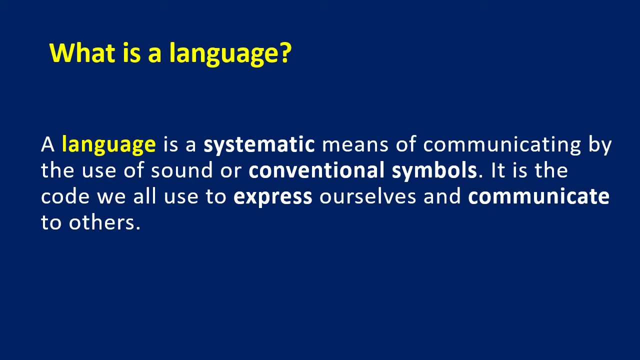 we need to get a good score, We need to get a good grasp of the mathematical language. Okay, first, what is a language? A language is a systematic means of communicating by the use of sound or conventional symbols. So, as you can see there, you also have symbols. 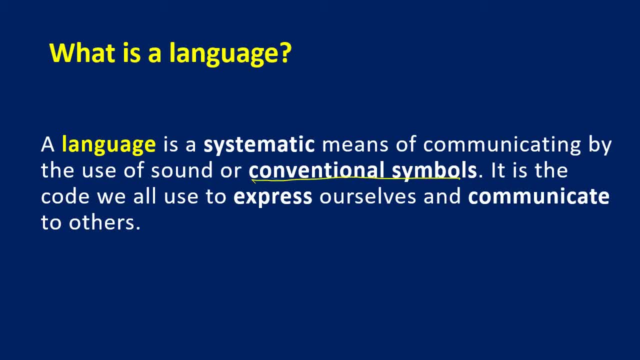 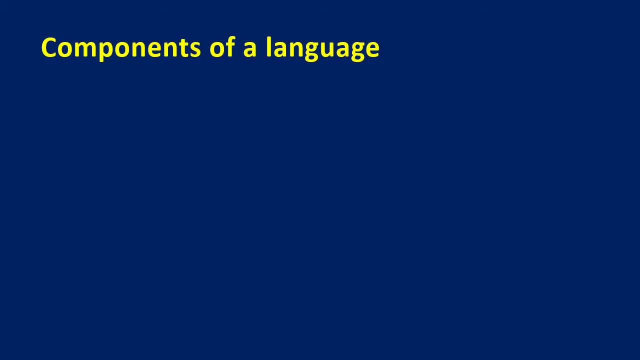 It is a code. It is the code we all use to express ourselves and communicate with others. Okay, what are the components of a language? So, for example, in the English language, we have vocabulary of symbols or words, grammar or rules of how the symbols are used. 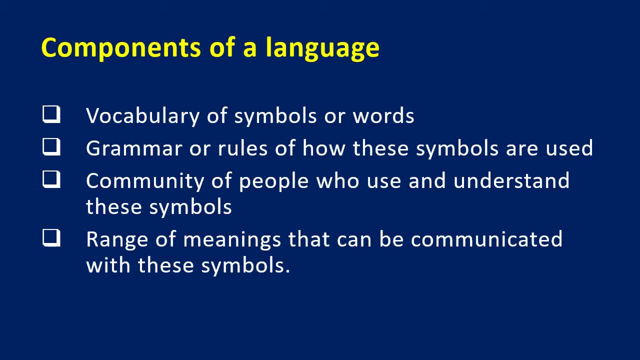 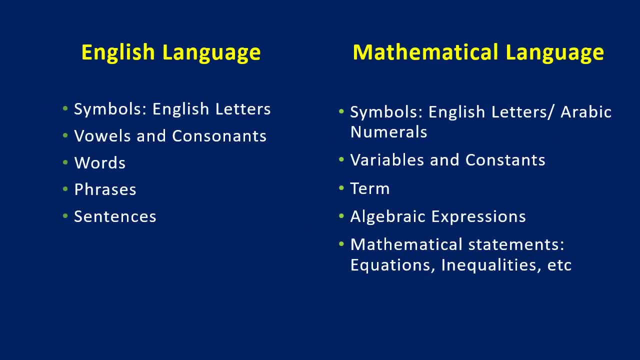 community of people who use and understand these symbols and the range of meanings that can be communicated with these symbols. So, for the English language, what are the symbols that we have? We have English letters For vowels and constants. we also have vowels and constants. 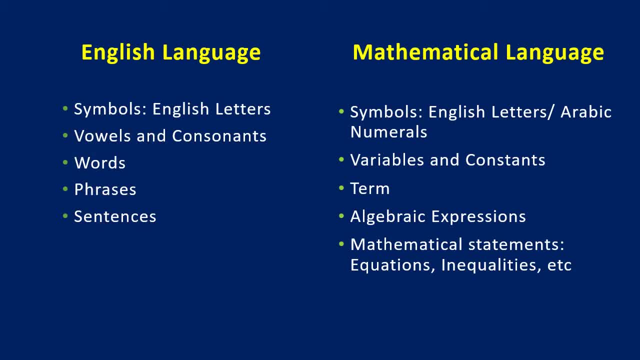 And then we have words, phrases and sentences. What are the mathematical counterpart of those? So the symbols in math would be the variables, or the English letters and some Arabic numerals, The vowels and consonants would be, And also the variables and constants. 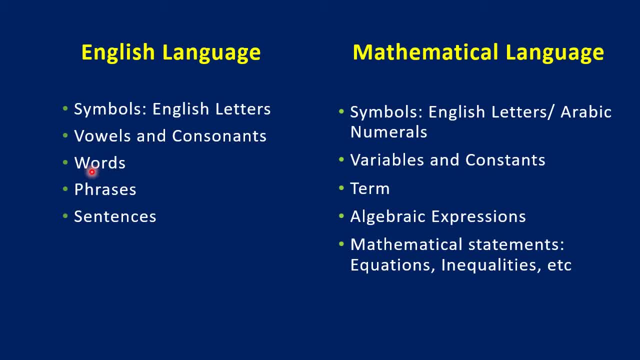 Okay, the words. So the words, the words in the English language. the counterpart in math would be the terms For the phrases- we have algebraic expressions and the counterpart of sentences would be mathematical statements like equations, inequalities and so on. 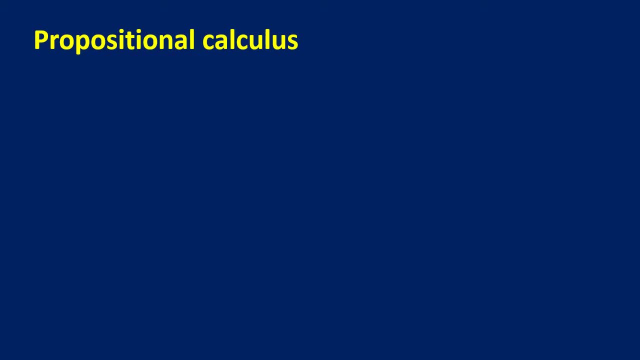 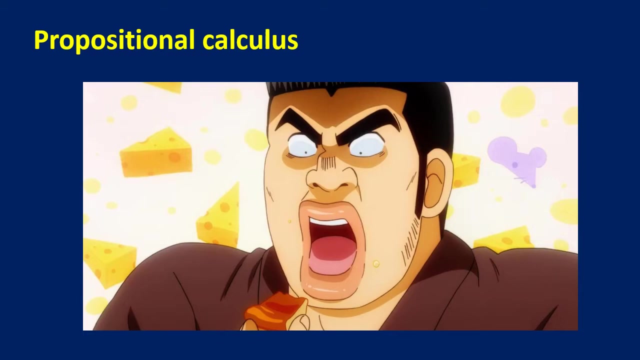 Okay, we will. as I have mentioned a while ago, we will be talking about propositional calculus. Now you might be distressed about this word, calculus. You might have that expression: what We're going to study, calculus. I did not sign up for this. 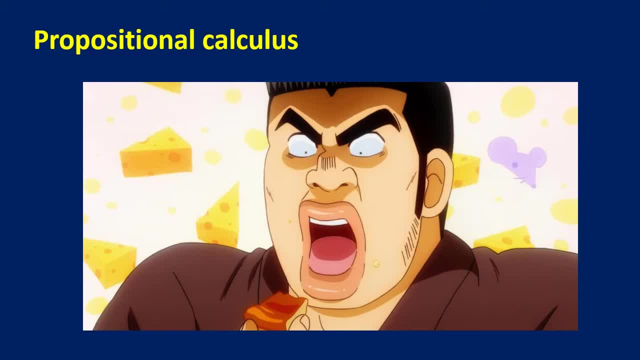 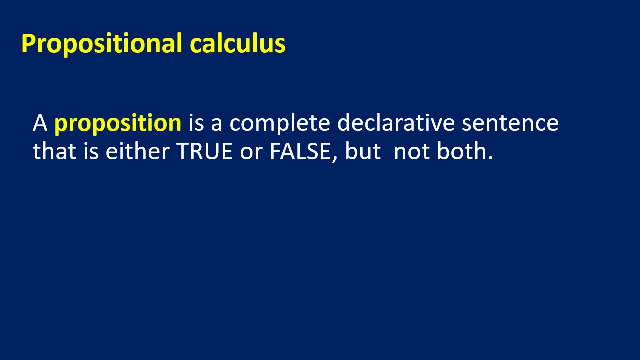 So it's okay. Take note: the term calculus here just means that we have it's a particular method or system of calculation or reasoning. First let us start with the definition of proposition. What is a proposition? A proposition is a complete declarative sentence. 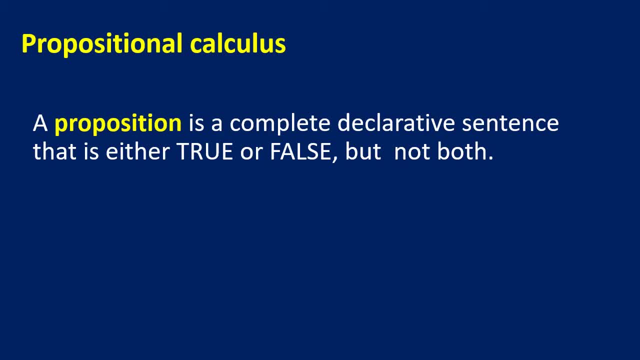 So let me just Let me just emphasize that it must be a declarative sentence Automatically. if it's not a declarative sentence, it's not a proposition. But of course, not all declarative sentences are propositions. A proposition is either true or false, but not both. 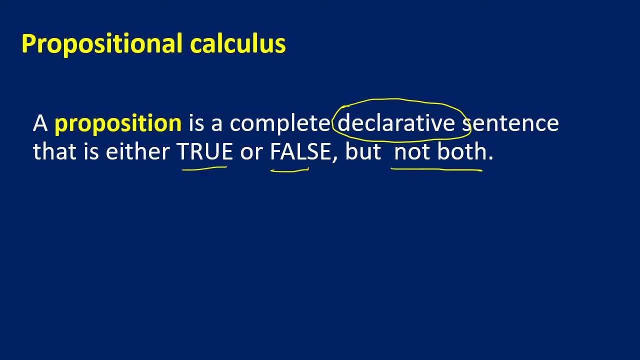 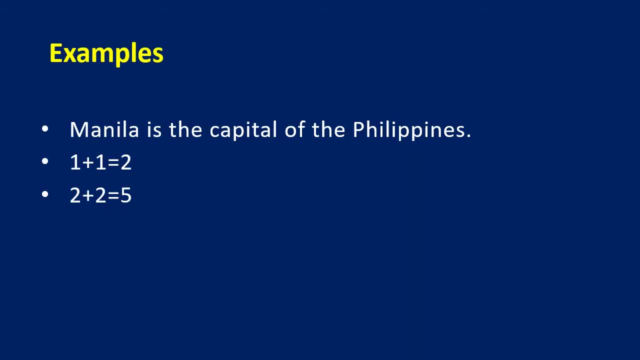 What do we mean by the statement that it cannot be both? So, for example, let's look at some examples of propositions. All right, so an example would be: Manila is the capital of the Philippines. We know that. that is true. 1 plus 1 equals 2, that is true. 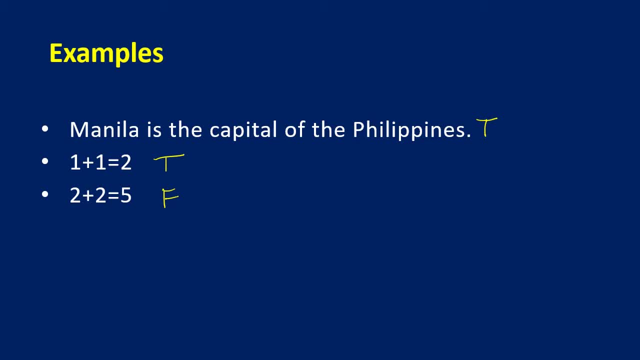 2 plus 2 equals 5, that is false. So these are all examples of propositions. What would be non-examples of propositions? For instance, we have wow, It's not a proposition simply because it's not a declarative. 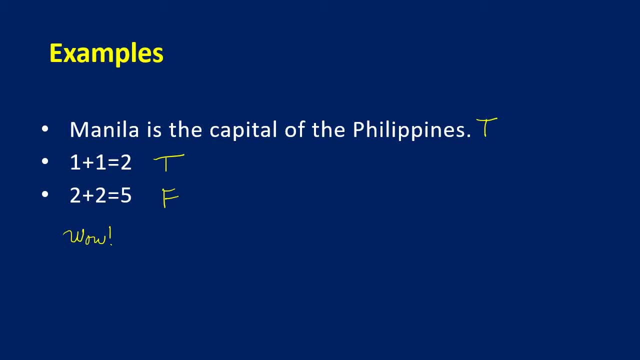 It's a declarative sentence, right? What about, let's say, Miss Universe 2020 is beautiful. It's a declarative sentence, right, But is it true or false? I guess most of you would say that this is true. 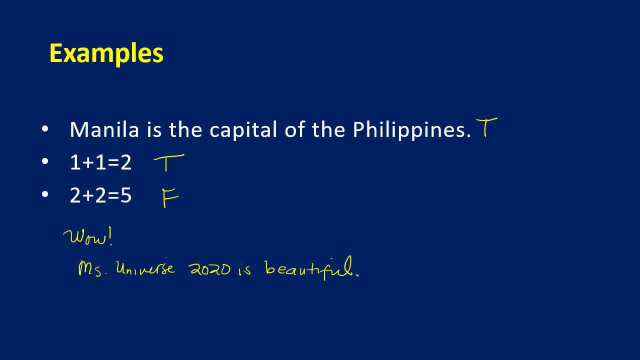 But take note that for this particular example, there are There are cultures that have different standards of beauty. So for one person- probably Miss Universe 2020,, I don't know who she is- she might be beautiful for him or her. 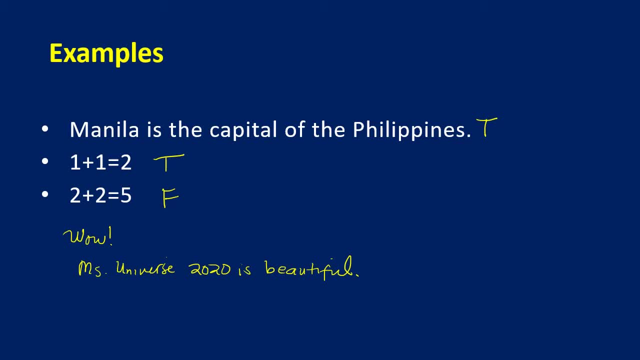 But for another person she might not be beautiful. So if in that's the case, this is not true, we cannot really say as a matter of fact that this is true. We cannot also say that it is false. So it's some sort of it depends. 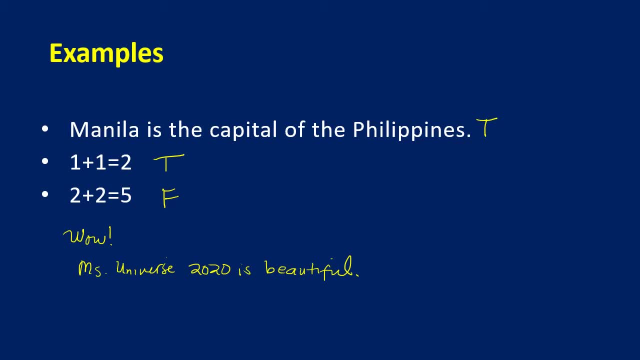 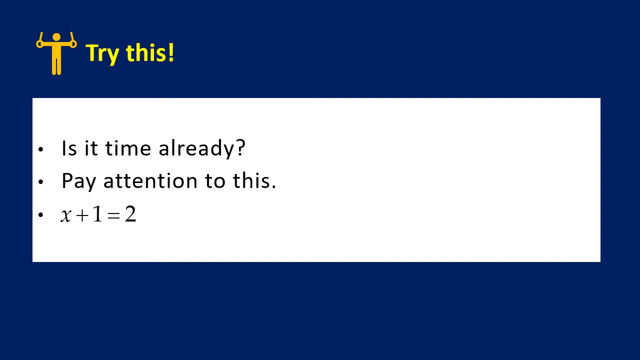 So statements were in. it depends. it's not a proposition, So these are not propositions. Okay, So is it time already? Is this a proposition? Of course, the answer is no, There's no question. here Are these Propositions. 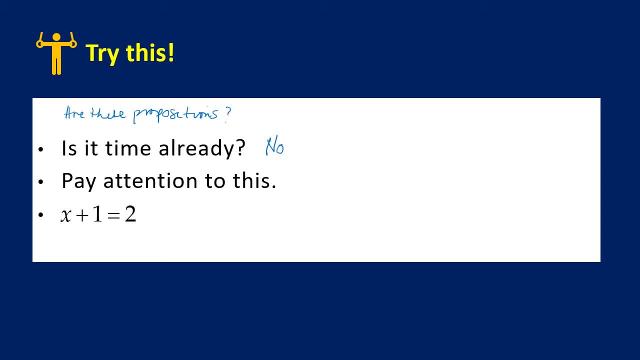 So is it time already? No, of course, because it is not a declarative sentence. Pay attention to this. It is a command. no, So it's not declarative. also, X plus one equals two. There you go. This is also not a proposition. 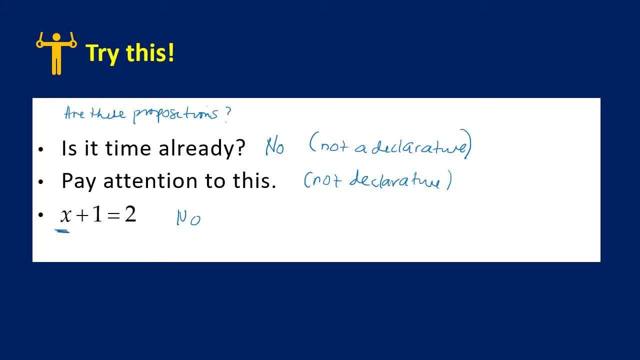 Why? Because we do not know the value of X, right? So if X is equal to one, then the statement is true, right? But if X is any number which is not equal to one, the statement would be false. So see, this is an example wherein it depends, right. 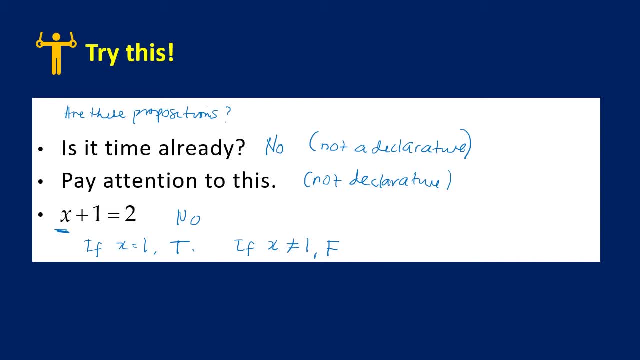 Just like in our previous example. So if it's, if you do not know, if you cannot say that it's true or false, it can be true or sometimes false. That is not a proposition, Okay. so what do we call those? true or false? 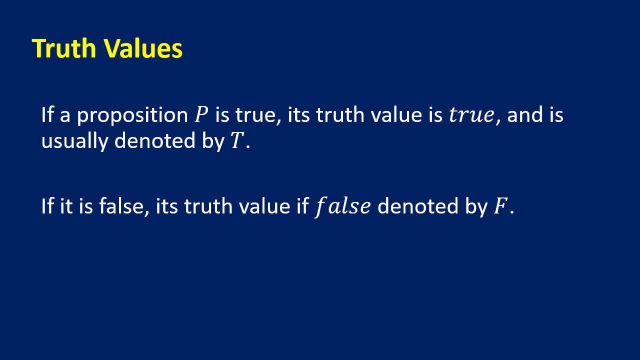 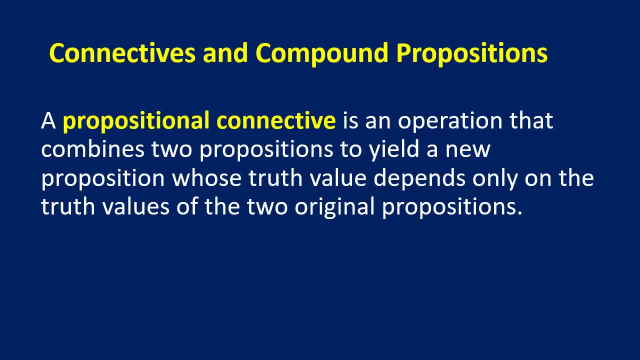 Okay, we say that those are the truth values of a proposition. So the truth values are either, of course, true or false. Okay, now we will discuss propositional connectives. What are propositional connectives? They're just like with numbers. 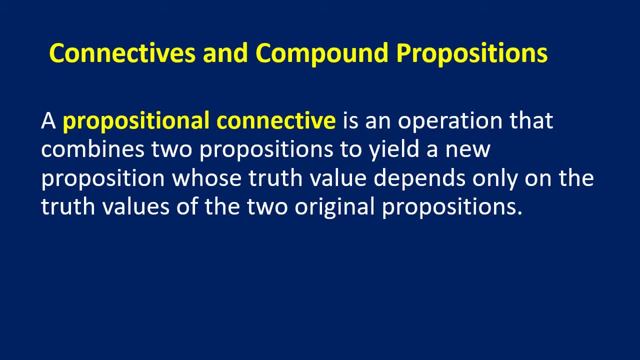 With numbers. you can join them right Using operations like addition, subtraction, multiplication, division. right, If you have a number, you add two numbers. Sorry, I'm sorry. If you have two numbers, you combine them using the operation of addition. 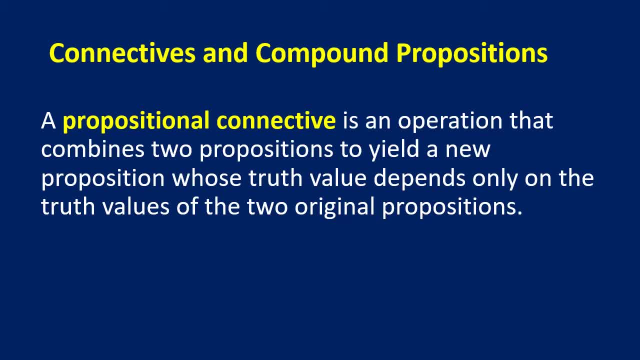 You yield another number correct. Or if you multiply two numbers you get another number as well. So also for propositions we can have some sort of operations okay with them. So yeah, they are really operations. So what happens here? 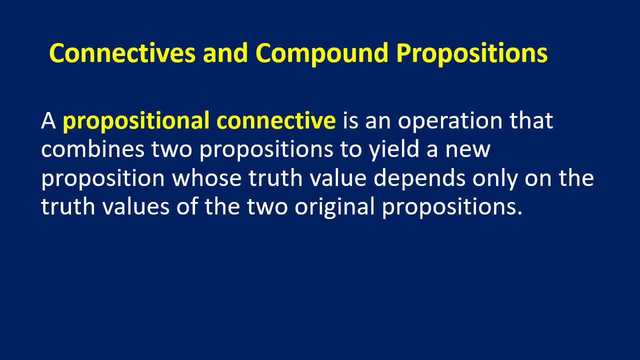 Is that you combine two propositions using this propositional connectives And the answer would be another proposition. Okay, and the value, the truth value of this, of this proposition, the resulting proposition, will depend on the truth values. It will depend on the truth values of the two original propositions. 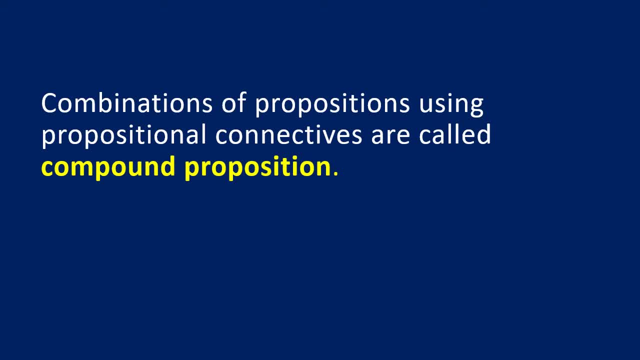 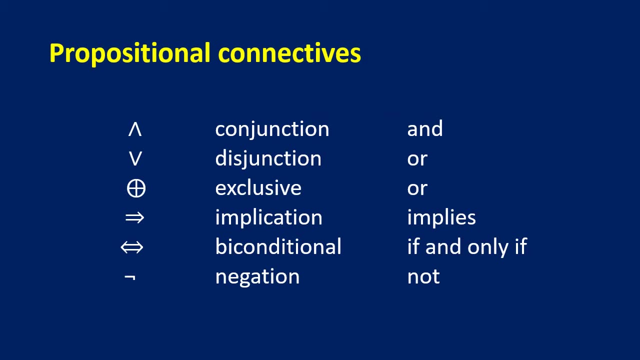 Okay, Take note that the combinations of propositions using propositional connectives are called compound propositions. So, just like with sentences, when you combine two sentences, right, you have compound sentences, All right. So here is just an overview of the propositional connectives that we would be discussing. 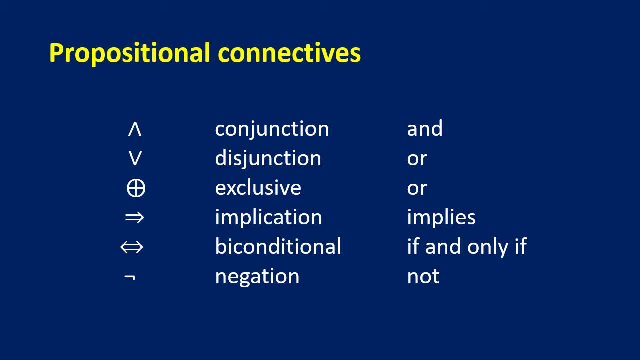 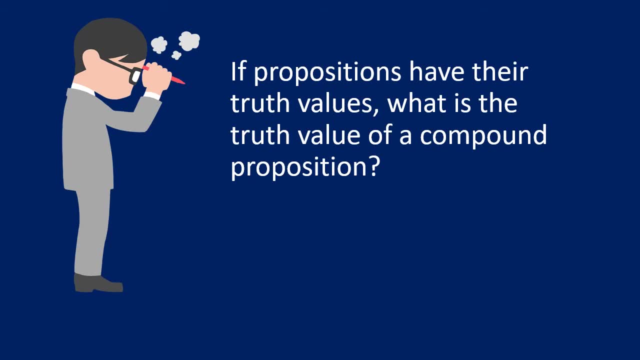 We have conjunction, disjunction, exclusive or implication, biconditional and deletion. Okay, Now note that if propositions have their truth values, what is the truth value of a compound proposition? Earlier I mentioned that the resulting proposition of two propositions connected by a propositional connective is a proposition right. 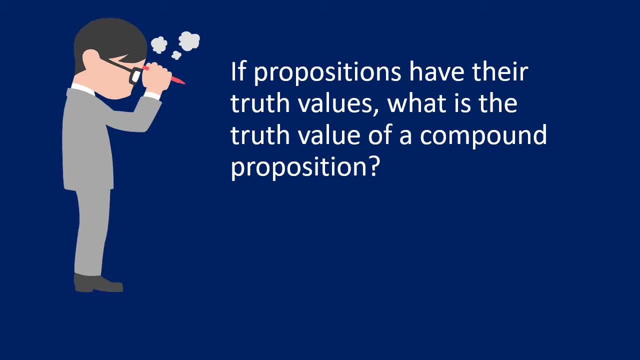 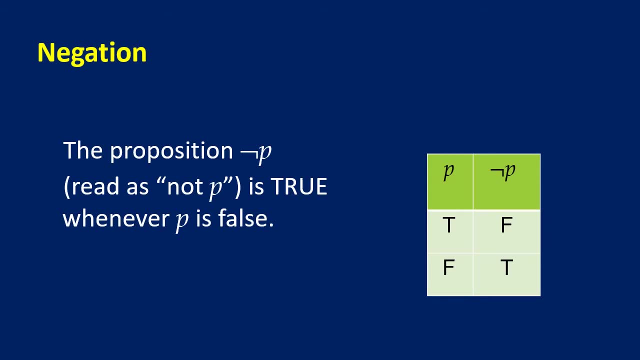 So therefore, it's either true or false, And the truth value would depend on the or two original propositions. Okay So let's discuss. Let's start first with the negation. The negation of a proposition is just the parang opposite. no, 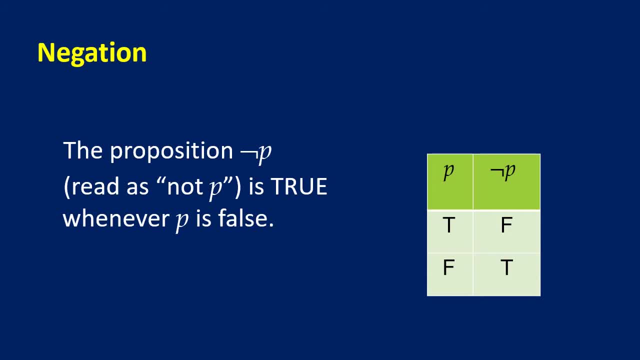 The proposition. this is read as not P, or sometimes we read this as the negation of P. It is true whenever P is false. So this would be the truth value. Take note that for P there are only two possibilities: It is either true or false. 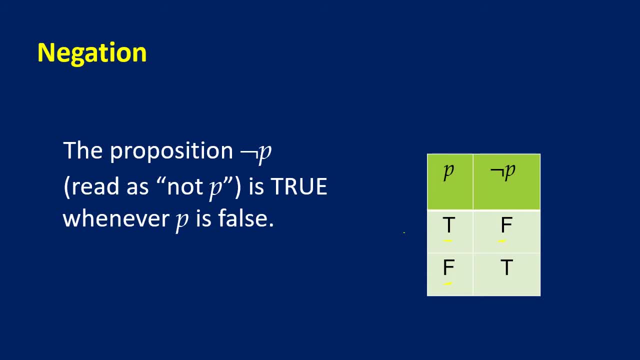 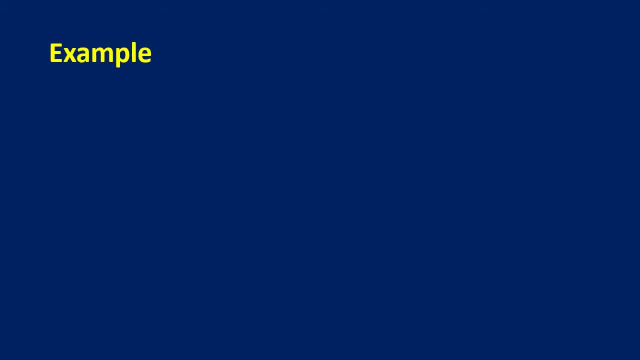 If P is true, of course its negation would be false. And if it is false, its negation would be true. Simple right. For example, the proposition is it will rain today. What would be the negation of this sentence? 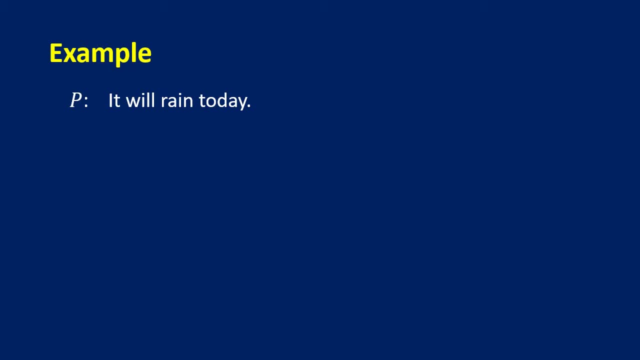 I'll just refer to it as sentence. What is the negation of this sentence? Of course it will not rain today. Another example: Shelby is hardworking. So the negation of the sentence is: Shelby is not hardworking. And lastly, you will pass this course. 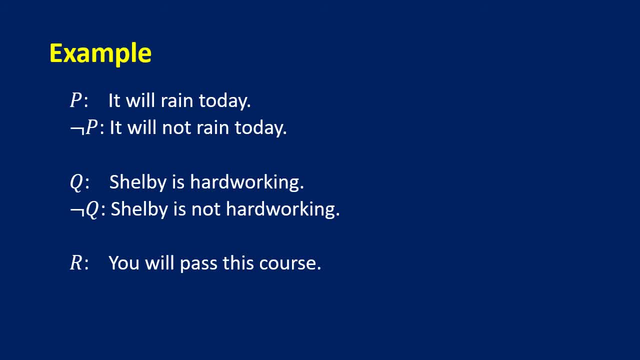 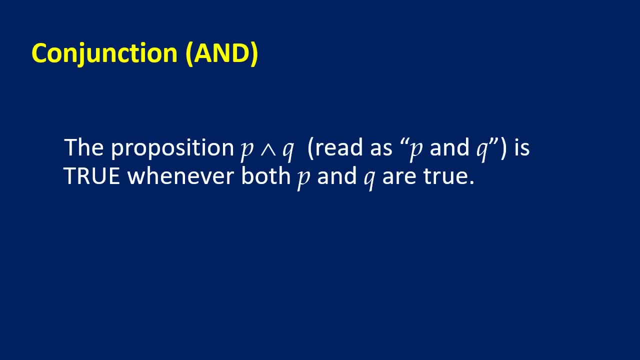 I am 100% sure that you will all pass this course. The negation of that sentence would be: you will not pass this course. Okay, So we just finished conjunction. Let's now go to the next connective. We have the conjunction and. 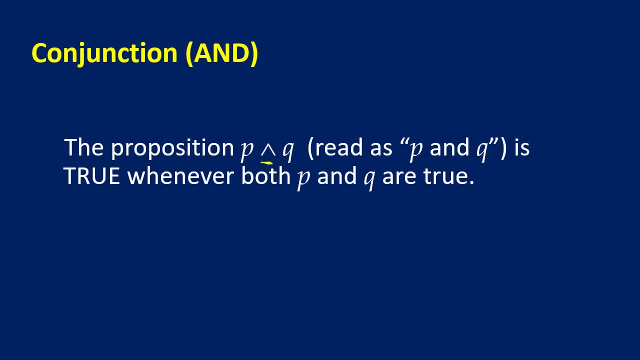 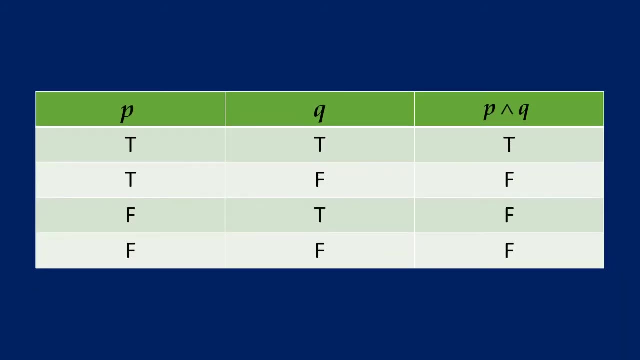 So this is the symbol for, and All right, P and Q is true whenever. take note that both P and Q must be true. All right. This is the truth. table of P and Q. So these are the four possibilities for P and Q. 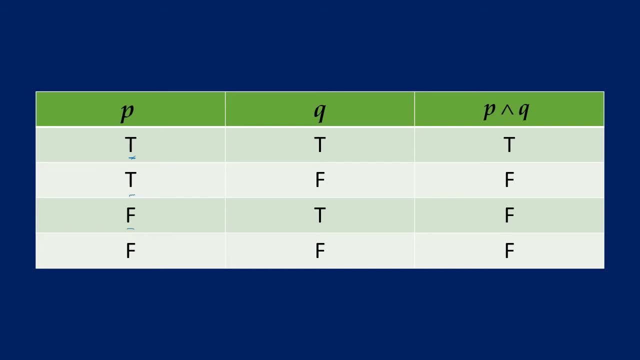 So P is either true or false, Right. Take note that what happens there, For P it's either true or false, but for Q- Right- It's either true or false. So it's like actually. So that's why you have that. 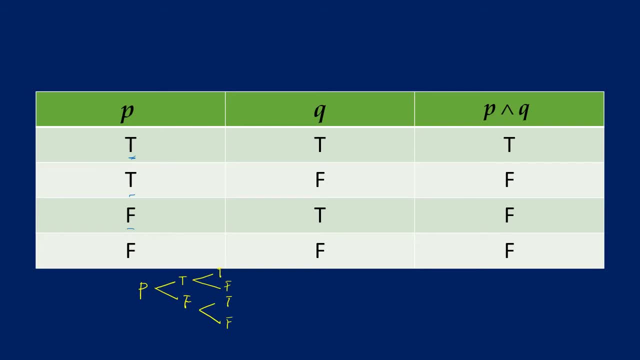 Okay, now let's look at the Okay this one. as you can notice, it is only true whenever both P and Q are true. For the rest of the values it's always false. Okay, Remember that P and Q is true whenever both P and Q must be. 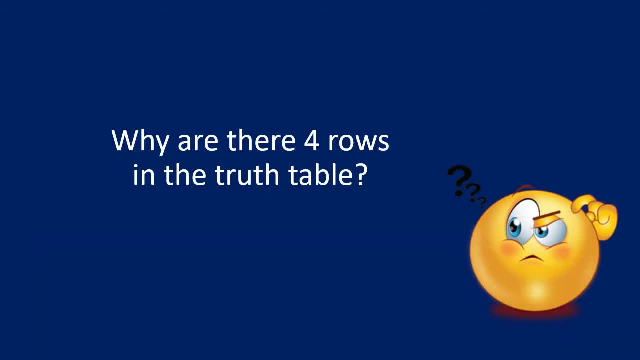 Whenever both statements are true. Okay, Actually, I already answered this question, right. Why are there four rows in the truth table? Anyway, before we go to that question, Let me just give an example of a statement. For example, I say July. 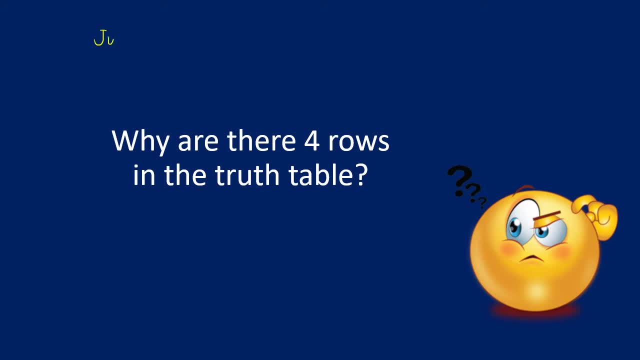 July 20.. 2020 is a Monday, And then Dr Song Song is male. Okay, let's just say that one. And then I connect this with the connector end. Okay, what would be the truth value of this sentence? 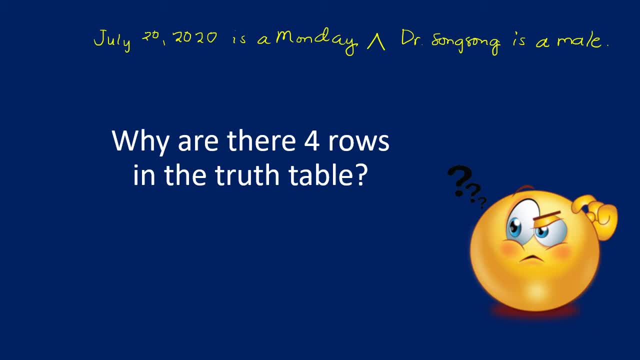 Is this true or false? The answer here is: this is false, right, Because although the first part- The first sentence- is true, But the second sentence- is the second component- is false. So that's why the entire thing is false. Okay, let's now go to this question. 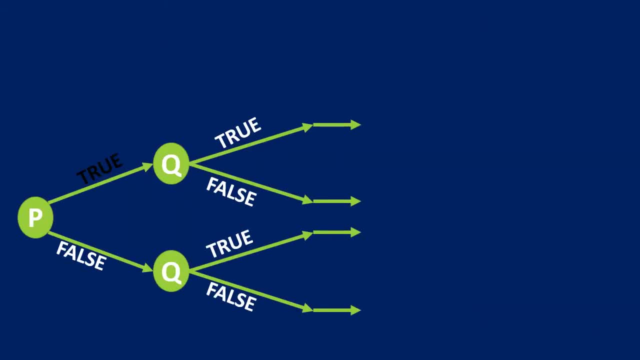 Why are there four rows in the truth table? I showed this a while ago, right, I just made it bigger. So for P we have two possibilities: True, false. And then for Q, For this part, Q is either true or false. 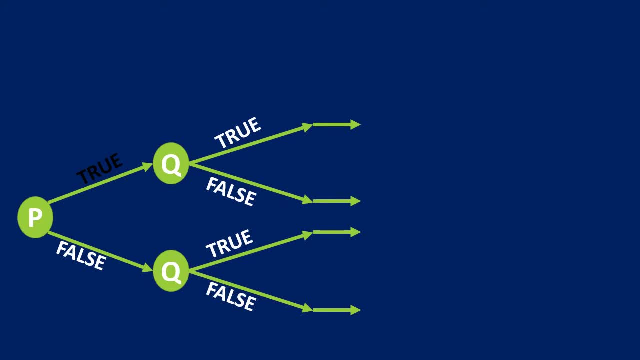 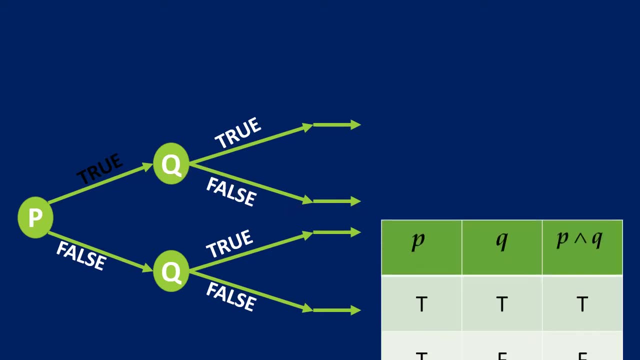 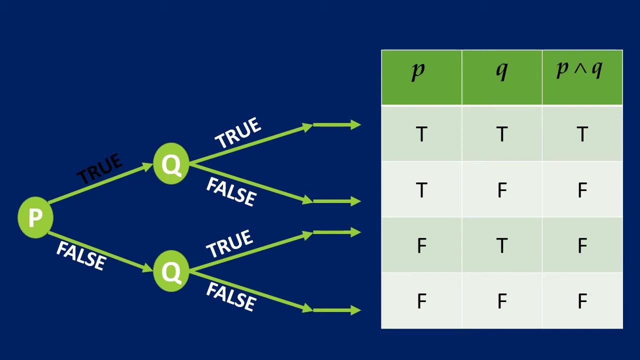 And then also for this one, Q is either true or false. So what will happen? We have four branches: correct, Correct. So there you go. So this is where P is true, Q is true. So you get this first row. 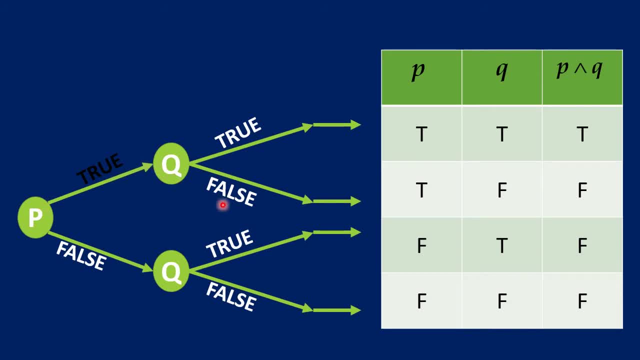 This one, This next branch, true. P is true, Q is false. So you get this row Right. This one: P is false, Q is true. You get the third row. And lastly, P and Q are both false. 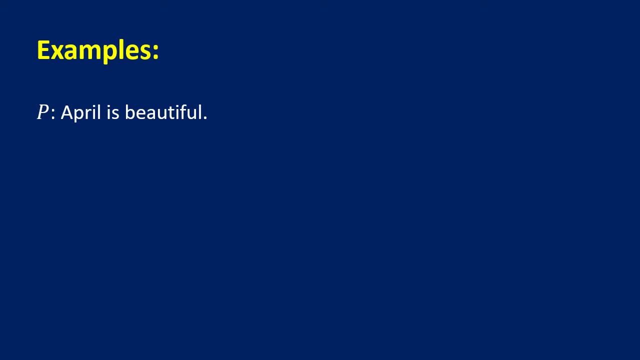 All right, Let's take a look at more examples. April is beautiful, Dominic is strong. Okay, we don't know the truth values of P and Q, But what would be the statement? P and Q? It is, April is beautiful And Dominic is strong. 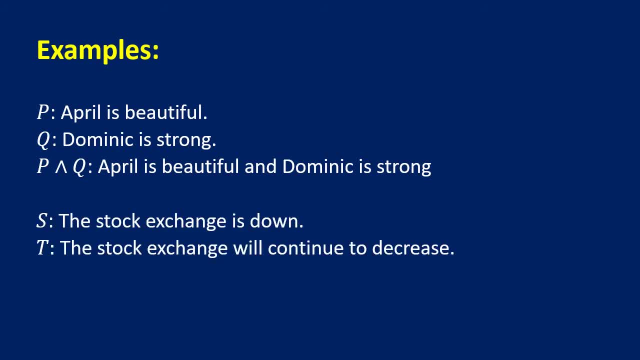 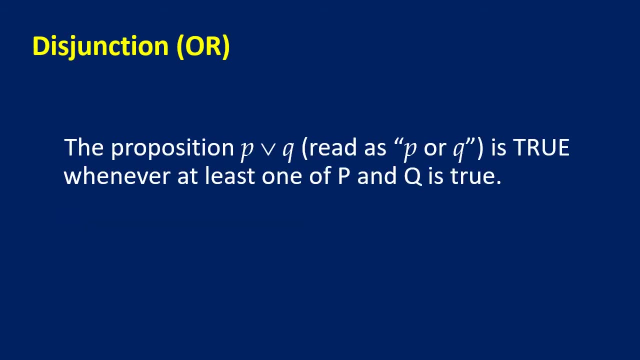 Next: the stock exchange is down, The stock exchange will continue to decrease. So when we combine them with the connector end, the stock exchange is down and it will continue to decrease. Let us now go to the next connector Disjunction, OR. 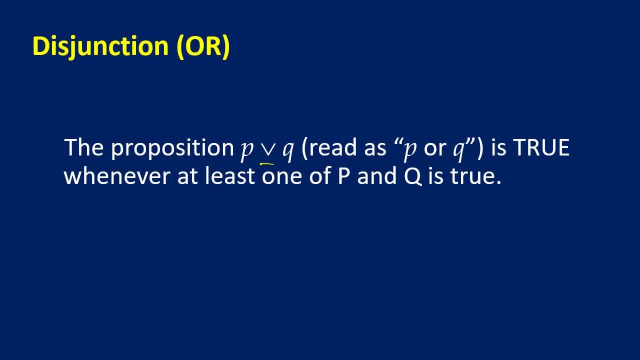 This is the symbol for OR. The proposition P or Q is true Whenever, at least one. You only need at least one of them to be true. Remember: for AND For, AND both must be true For it to be true. 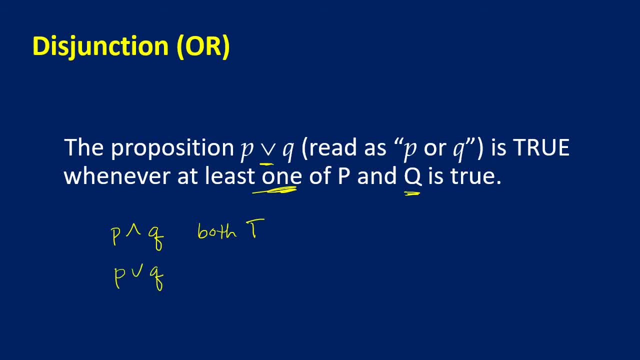 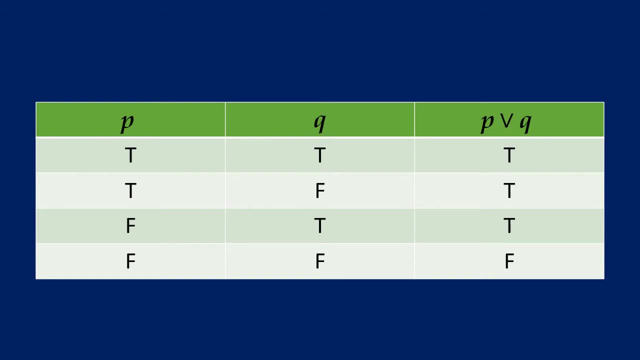 For P or Q, you only need at least one. Okay, So this is now the truth table of P or Q. As you can see, here We have these values right: P and Q. For P or Q, everything is true. 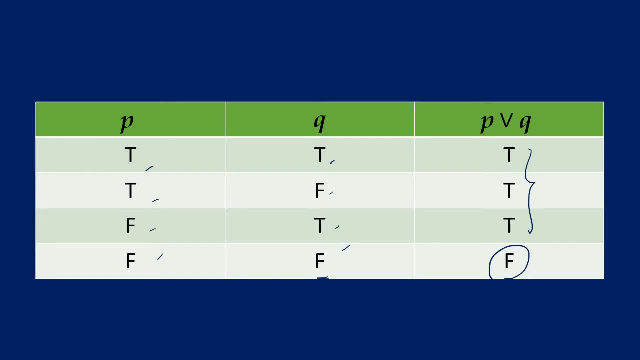 Except for the last row, Because none of P nor Q are true. Okay, So remember, remember, we will. This is important for P or Q. If you get at least one to be true, automatically the entire statement is already true. 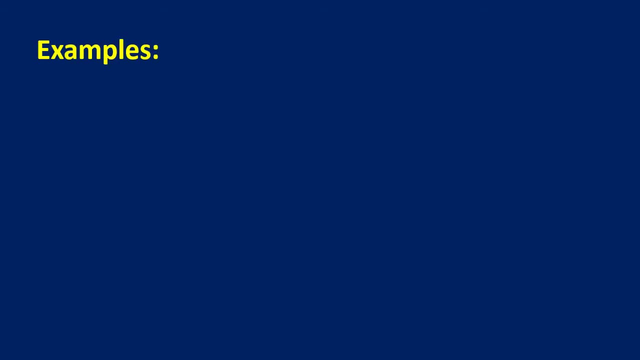 If it's connected by: OR. Okay Examples: This lesson is interesting. Q- the lesson is easy. What is the statement? P or Q? This lesson is interesting or it is easy. Next, I want to take a diet. That's S. 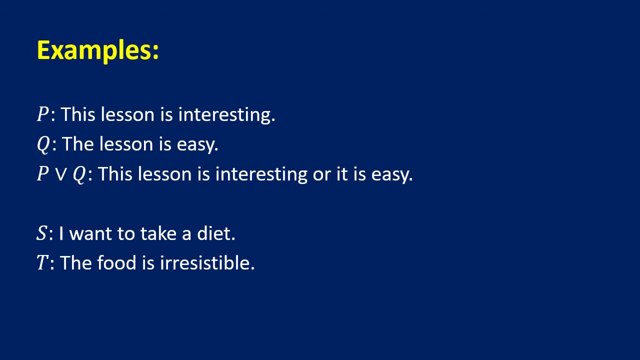 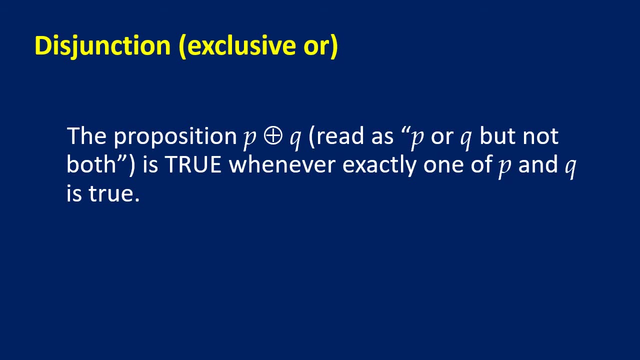 T- the food is irresistible. What is now the statement S or T- I want to take a diet or the food is irresistible, Okay. Next We have the exclusive or the disjunction exclusive, or. take note, It's just not, or? 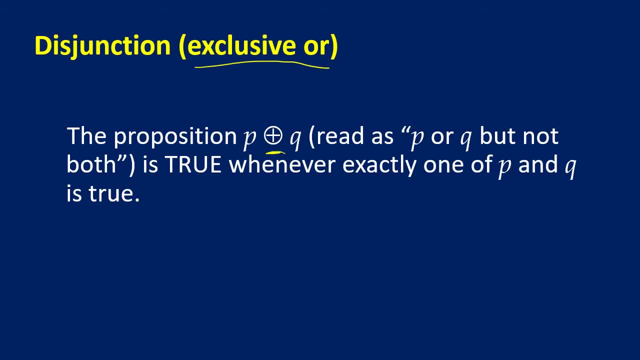 Okay, The symbol here is different, So how do you need this? P or Q, but not both. It is true whenever- take note, Exactly one of P and Q is true. Remember what is the difference with the OR, like that For that. it is true whenever at least one. 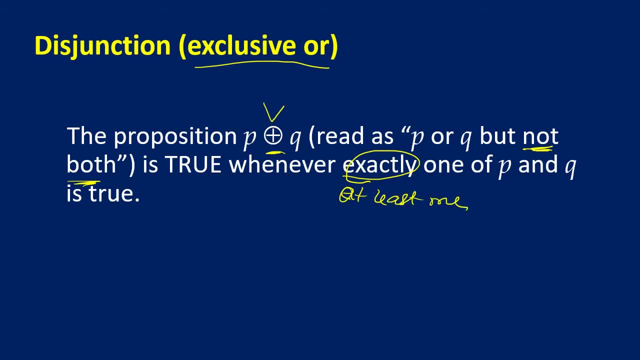 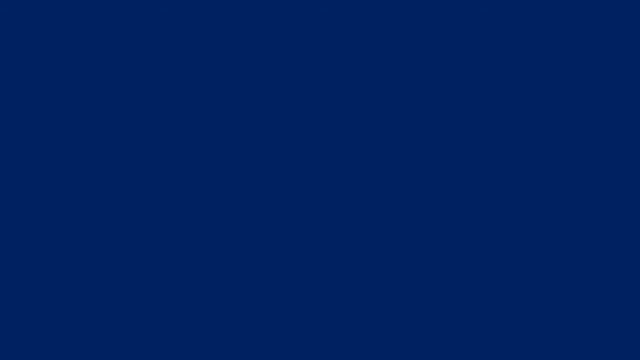 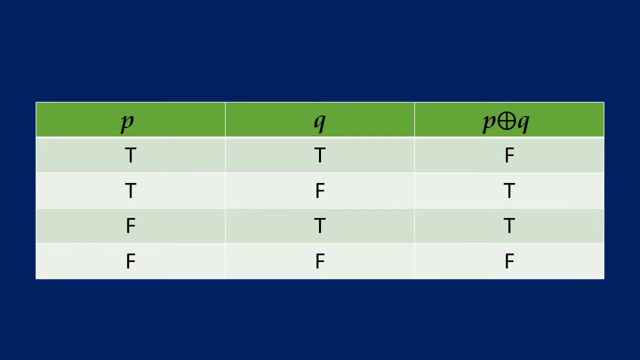 At least one, Meaning to say it can be one or two, Two of them, Right. So that means take a look at the truth table. Look at this. for the first row, It is false because you have both of them are true for it to be true. 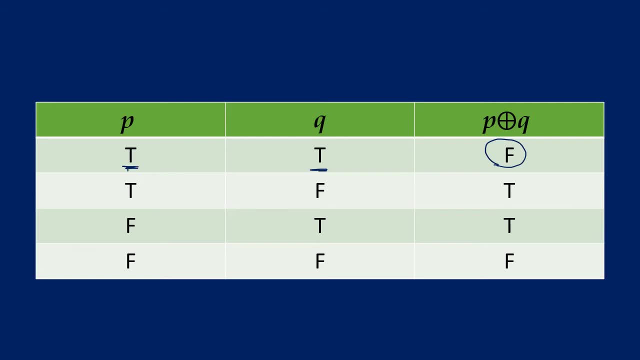 You need exactly one to be true for this. It is true because you have only one T. You have only one T, Okay, And this one, of course. it's false because both of them are false. Remember, you need exactly. 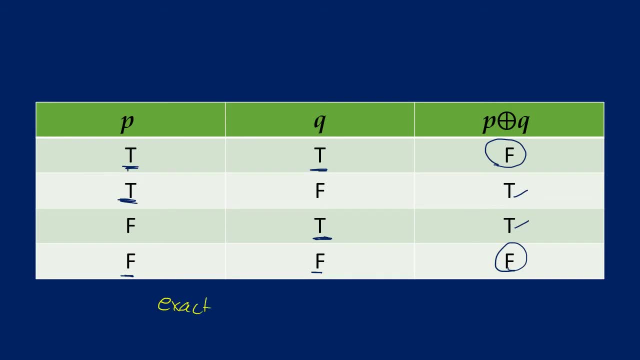 You need exactly one T. Let me just write the truth table. if it's OR, What's the difference class For OR, like that, this row would be true, correct? This is true. This is true. This is false. So this row here, the first row, is the difference. 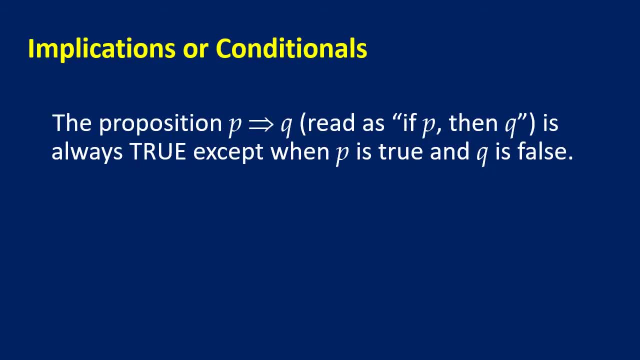 All right. Next, let's look at implication, Implications or conditionals. This is read: if P, then Q, The proposition, if P, then Q is always true. So remember for the other connectives that we discussed, we're always telling you when is it true. 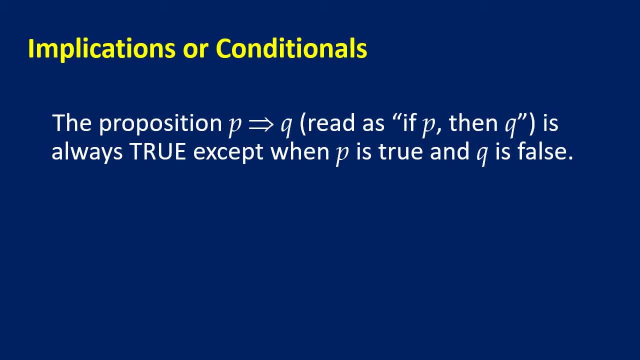 Right, We're just giving you the conditions for it to be true. But for this implication it is always true, Except there is only one case wherein it will be false. It will be false when P is true and Q is false. Okay, 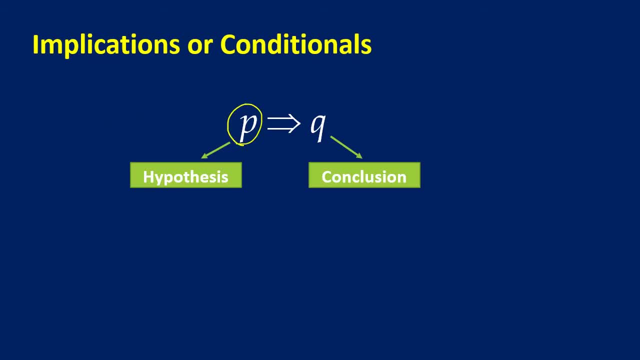 Now take note for implications. You call this. I don't want you to think of it as P, Q, something like that, Because P and Q they're just, you know, letters. They can be anything, Okay. So what I want you to do? 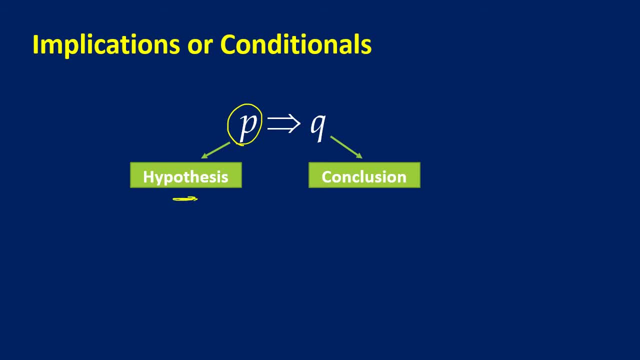 Okay, So the first part that appears there, that is called the hypothesis, And the second part is called the conclusion. I want to show you why. Remember, it is false only when the premise or the hypothesis- Let's call that the hypothesis. 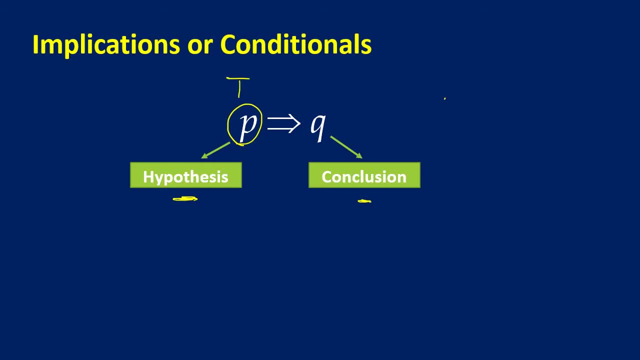 When the hypothesis is true but the conclusion is false, It will be false there. Okay, I want to show you an example. For instance, let's say, if you get A four In Gemat MW, I will give you. 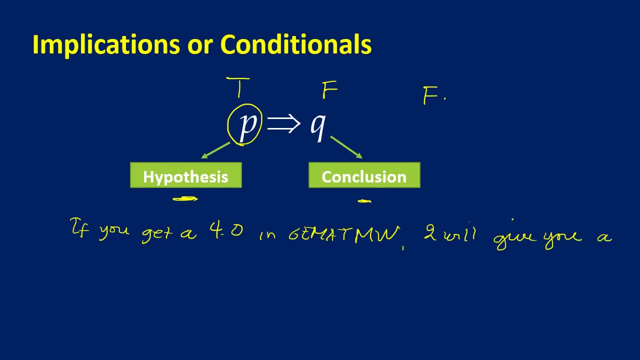 For example, I'm your mom, I will give you a new cell phone. Okay, Let's say, she promised you that If you get a four In Gemat MW, I will give you a new cell phone. Now, suppose that. 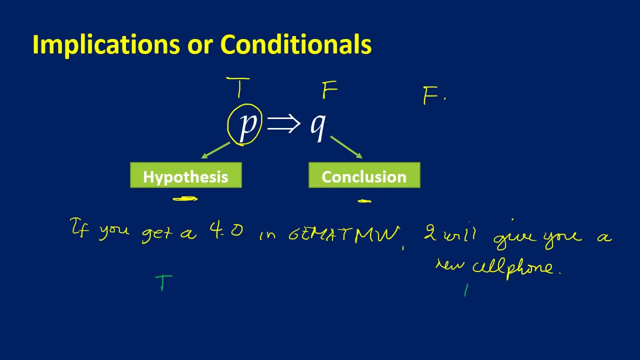 You got a four Right, And then she gave you a new cell phone. So this part here is true. Okay, When you get mad at her, No Right, You're still happy. Next Suppose You did not get a four. 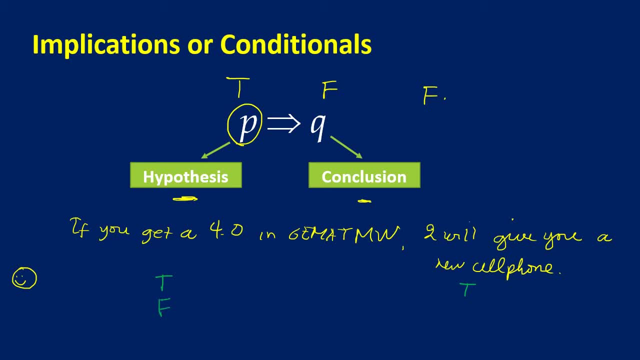 So this part here is false. You did not get a four, But your mom saw your effort, So She still gave you a new cell phone. Will you be happy? Of course you will be super duper happy, Right, Because even if you did not meet the condition, 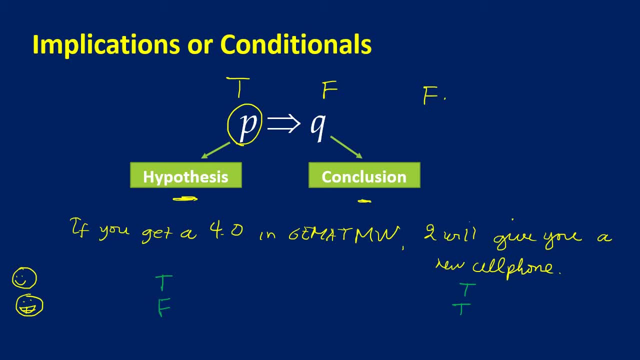 So that's a grin. Okay, Even if you did not meet the condition, She- just she- still gave you a new cell phone. All right, Now suppose Again: you did not get a, You did not get a four, And of course she did not give you a new cell phone. 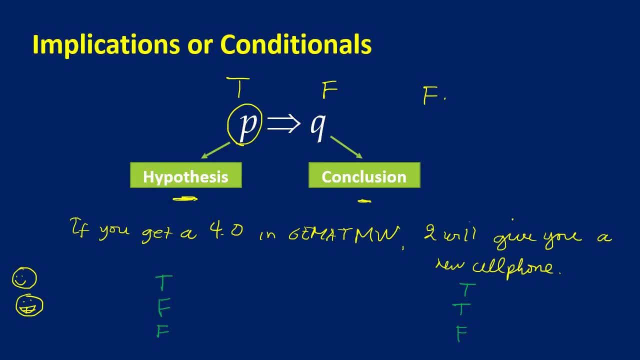 So this is false. Will you be mad at her? Do you have the right to be mad at her? Of course not. You should not be mad at that. But you're not happy because you did not get a new cell phone. But the point is, you have no right to be mad. 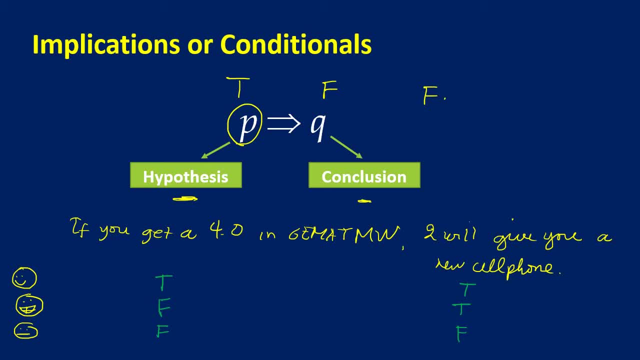 When will you be mad at her? When? When you got a four but she did not give you a new cell phone? So this part here. The hypothesis is true. You met the condition, right, The hypothesis is true, But the conclusion was false. 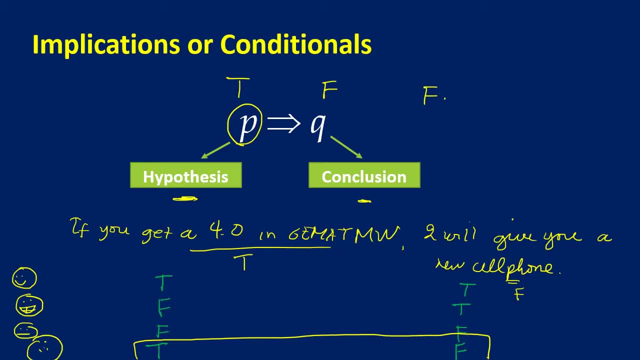 This is the only time that You can be mad at her Right. So the reason why I showed this to you so that because when I was your age, I was always thinking: why is it that special that if the hypothesis is true and the conclusion is false, then it will only be the case when the 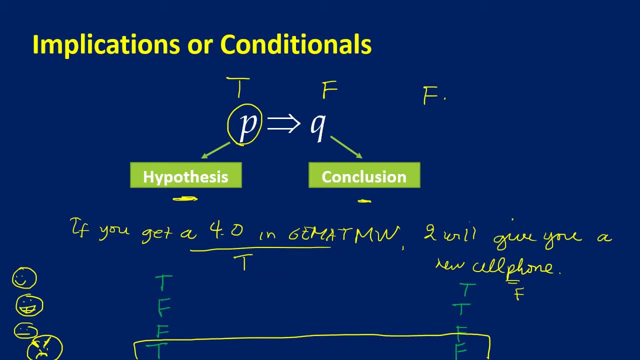 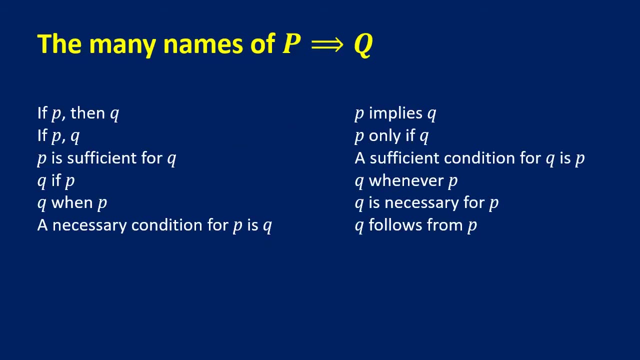 the entire implication would be false, right? So if, if something like this happens, if the hypothesis is true, but the conclusion is false, that would make the person who said the statement a liar Right? Um, we will go back to the to the truth table. 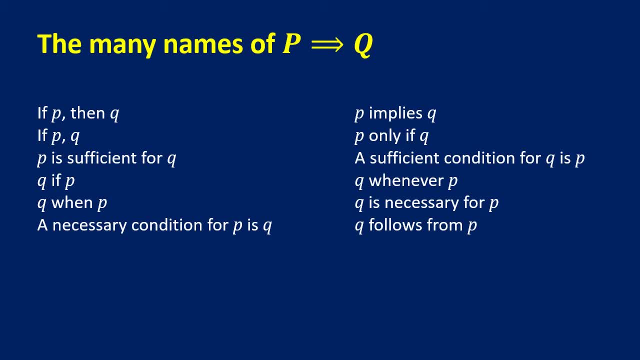 Anyway, these are the many names of if, P, then Q, So, as you can see, there are a lot OK, so take note that if, if, if the statement is starting with if, The, the, the, the part that appears there would be your hypothesis. 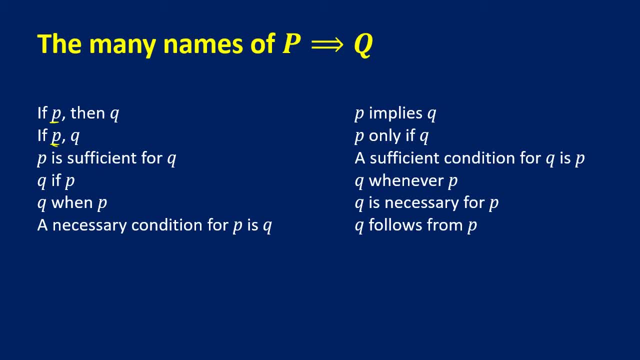 And then the second part would be the conclusion. Also, it can be said that P is sufficient for Q. Take note that this one Q if P, it will be reversed Because, after the word, if you, after the word, if, that will be always your premise. 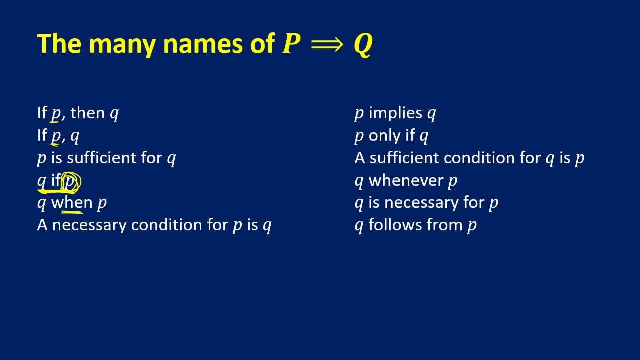 Ito rin Q when. P when is the same as if Right. So this is your premise. Unnecessary condition for P is Q. Actually, ito yung medyo nakakalito. This too Necessary and itong sufficient condition. 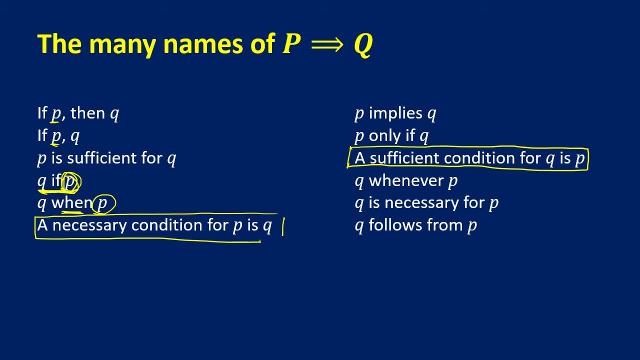 So even for me- actually, you don't have to memorize this. Whenever I see this, I just go back to the table And then this one: the whenever, Q, whenever P is almost the same as Q when P, like it's actually the same. 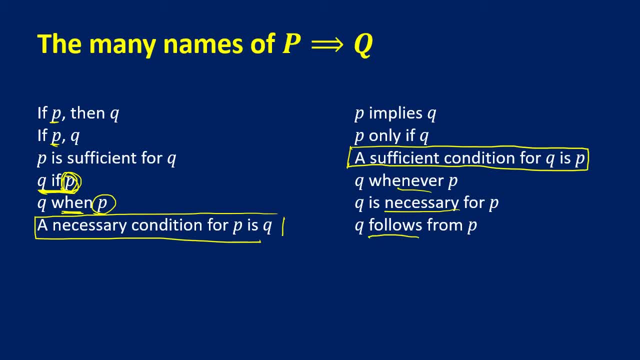 And this one Q is necessary, Q follows. So remember, whenever you have necessarily follows, then that would be na ma-reliberts. OK, so you start with this part. That's the premise And this is the conclusion. OK, anyway, this one lang. 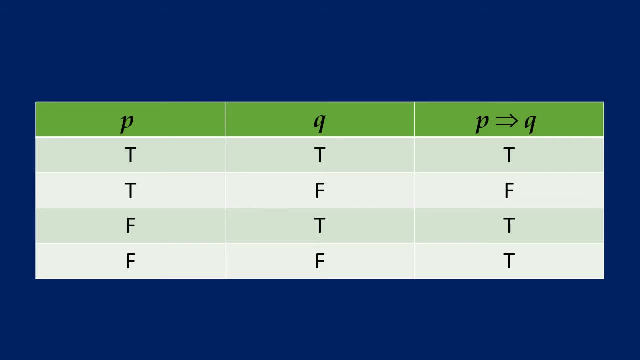 I'm just giving you the truth table for the for the implication if E then Q, And then this is the part that I I told you na. this is the only row wherein you will get a false. for if P, then Q, when the premise is true but the conclusion is false. 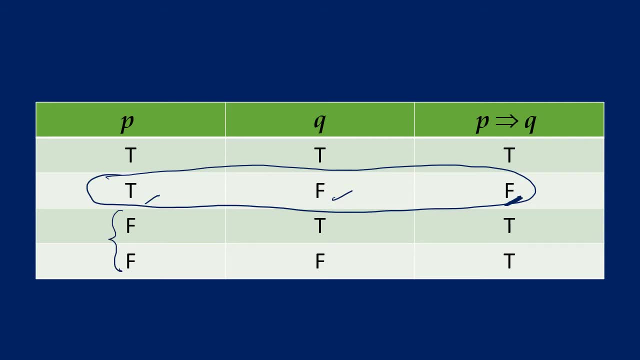 And take note also. it's worth mentioning also that automatically if the premise is false, it doesn't matter if the conclusion is true or false. Automatic The sentence would be true. OK, for example, let's say: I have Um. let's say Tuterte. 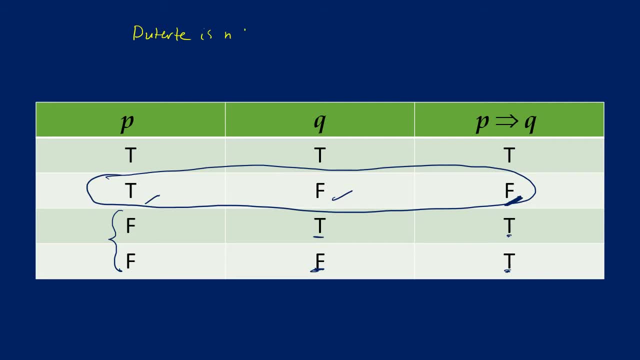 is not. Tuterte is not true, Tuterte is not true, Tuterte is not true. But if it's not the president Of the Philippines- That's my premise- then the third day is not the president of the Philippines. 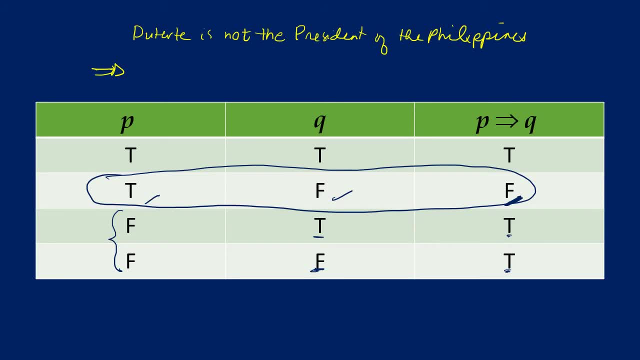 Then I am going To run for vice president. let's say, if the third day is not the president of the Philippines, I am going to run for vice president. Now take note that The first part, this one, This is false right. 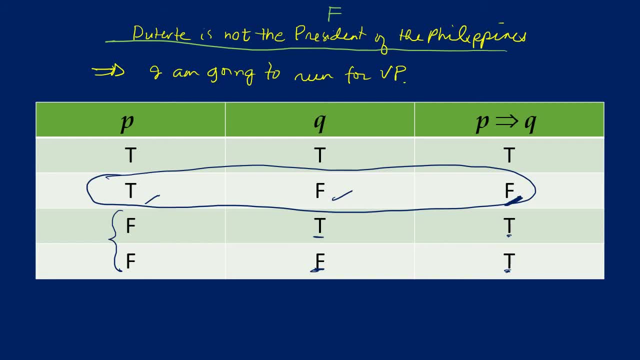 It is not true that the third day is not the president of the Philippines, because he actually is. so it doesn't matter what the truth value of the conclusion right, This makes this one. It doesn't matter, OK, whether it's true or false. 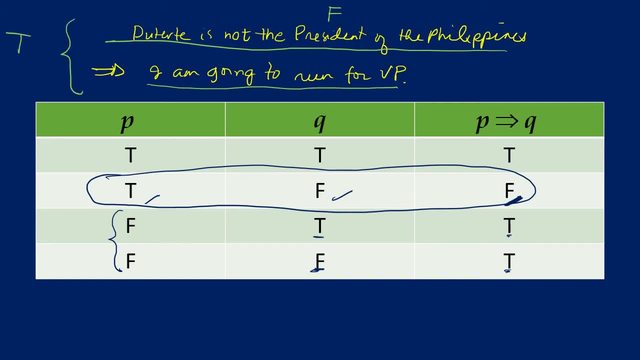 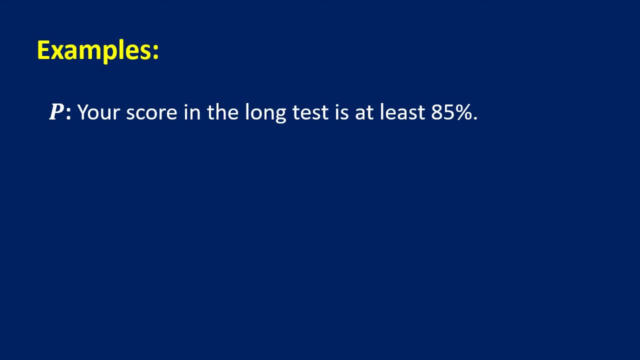 But the point is, this entire statement is true, Understand. OK, Let's have some examples. P- your score in the long test is at least 85 percent. Q- your teacher will buy you some pizza. The implication if P, then Q is: 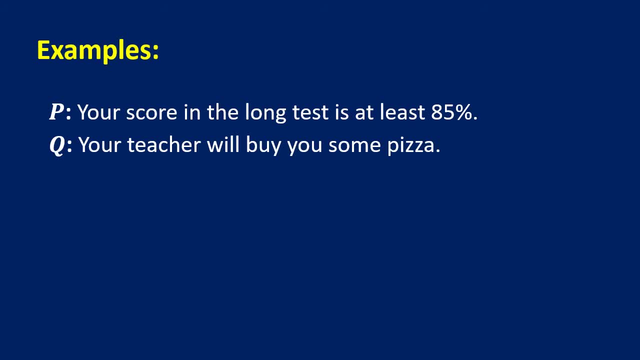 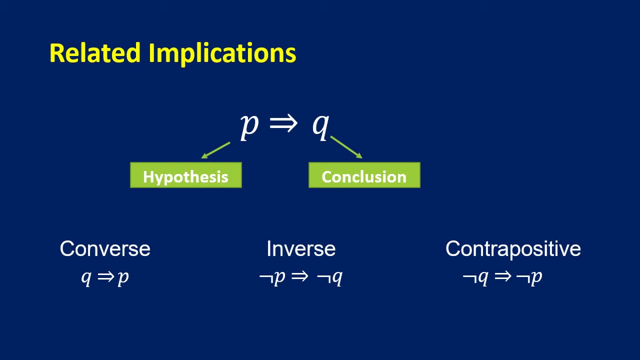 If your score in the long test is at least 85 percent, Then your teacher will buy you some pizza. Anyway, let us now look at some related implications. So we started with this one, the implication: If P, then Q. remember, this is the hypothesis and this is the conclusion. 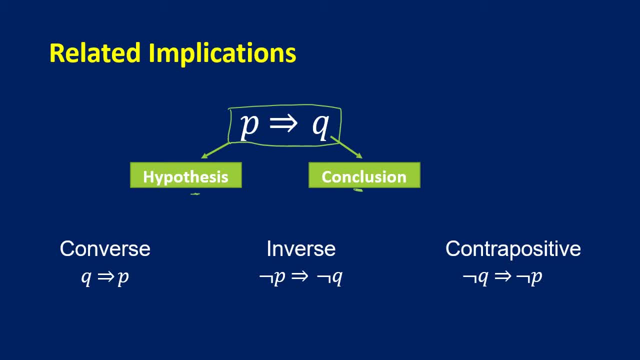 We have three related implications. The first one is the converse. What happens with the converse? For the converse, What happens is that the hypothesis and the conclusions got interchanged right. Interchange the premise and conclusion For the inverse. What happens for the inverse? 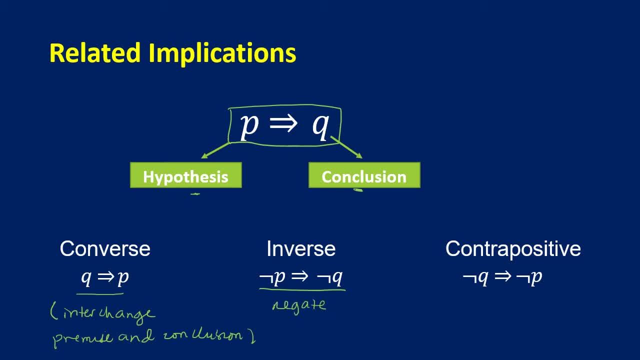 So what happens is you just negate, negate both premise and conclusion. right For the contrapositive. the contrapositive is actually what? The contrapositive? if you will look at this, what happens to this? What is your relation with this one? 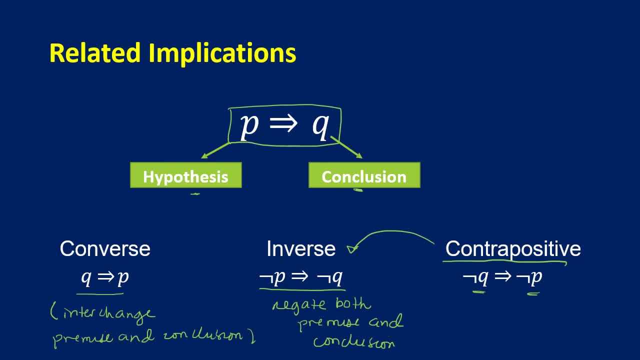 The contrapositive. what happened? It's the converse. So the contrapositive is the contrapositive of the inverse right. So what happened? It's like you negate it, you get the inverse first right. You negate both of this, but then you switch. understand. 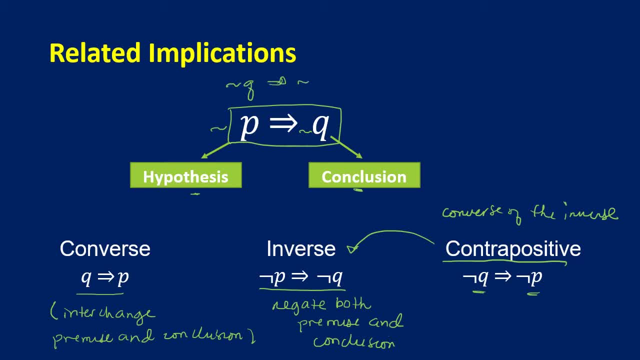 And then you switch: That is the, that is the contrapositive. So meaning to say: remember to get the contrapositive, um, the new. so wait, let, let me just write that again: P, then Q. 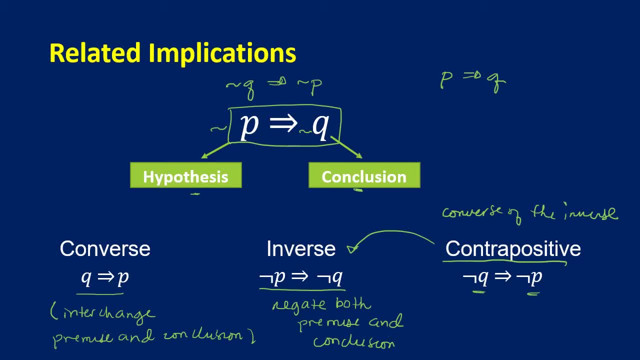 So to get the contrapositive. the new premise is the negation of the conclusion and the new hypothesis. Sorry, I'm always referring to hypothesis as premise. same lang din nga. Again, the new premise is the negation of the original conclusion and the new 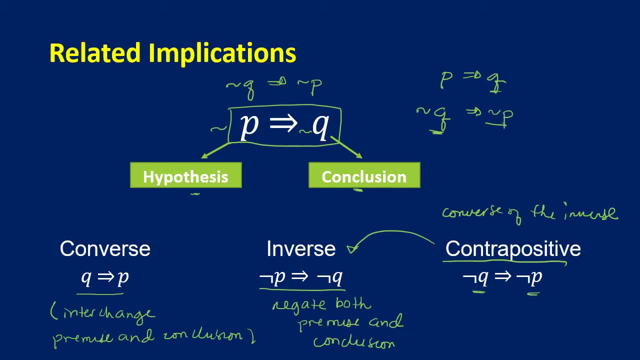 conclusion is the negation of the original Premise. maybe I should write this that like that understand OK? so it's very important that you memorize contrapositive by how to form the contrapositive. I will show you later why it's very important. 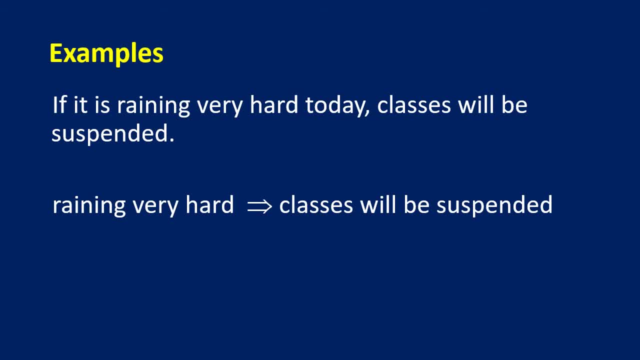 Example: if it is raining hard today, classes would be suspended. Of course, now during the pandemic, even if it's raining very hard, wala nang suspension of classes, because we are still doing online, So anyway. so suppose that we are in the 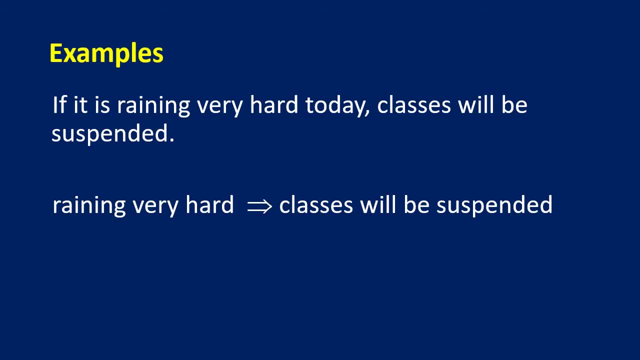 in the old normal those days when this is true. If it is raining very hard today, classes will be suspended. So the if you write it in this way, the premise is: it's raining very hard and the conclusion is classes will be suspended. 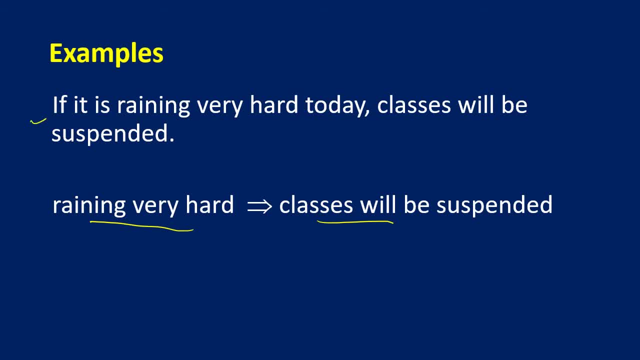 So take note, class, that it's important that if you're given a sentence like this, you should be able to know which one is the premise And which one is the conclusion. OK, now, what would be? so? this is the original, the statement that we had earlier. 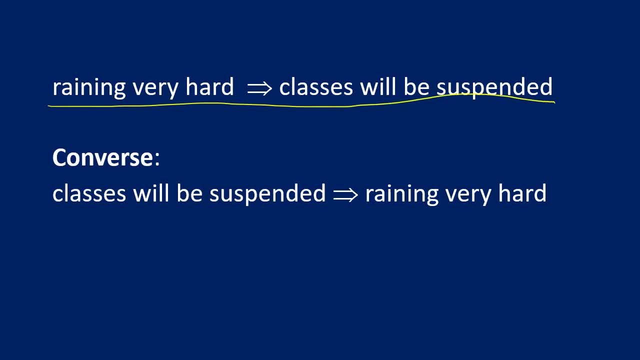 OK, it's raining very hard, then classes will be suspended. How do you form the converse? You just interchange the hypothesis in the conclusion. So that's why classes are actually. let's turn this to: if classes are suspended, Then it must be raining very hard. 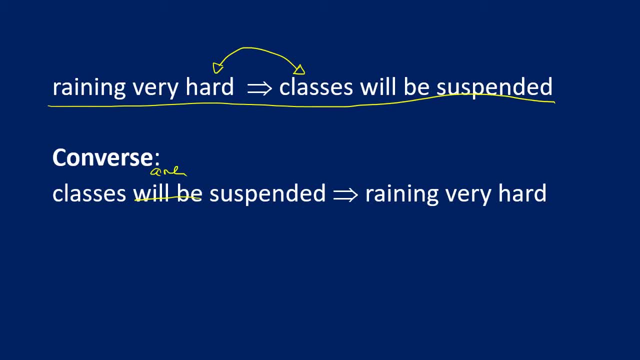 That is the converse of that statement. Understand So, for example, another example. let's say: if I, if, if I get bored, then I will go to the mall. What is the converse of that statement? If I go to the mall? 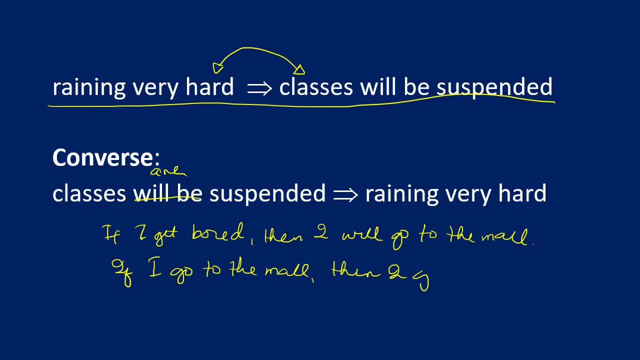 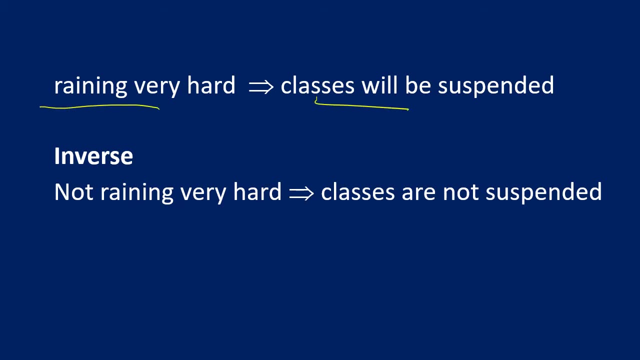 then I got bored, right, Right, OK, Let's look at the inverse. So remember how do you form the inverse of the original statement? You just get the negation. This is the wiggle part. Sometimes I'm using this: 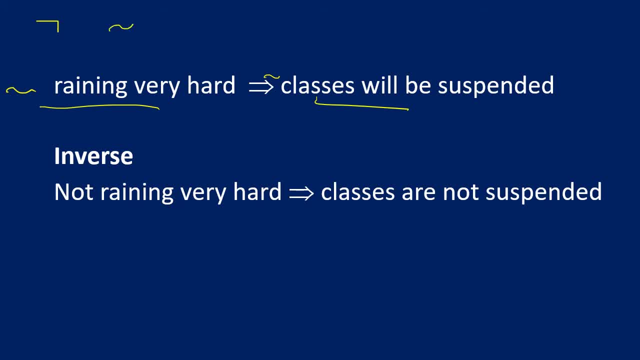 but most of the time I'm using this for the negation. So the inverse would be: if it's not raining very hard, then classes are not suspended. And lastly, we have the contapositive. So how do you form the contapositive? 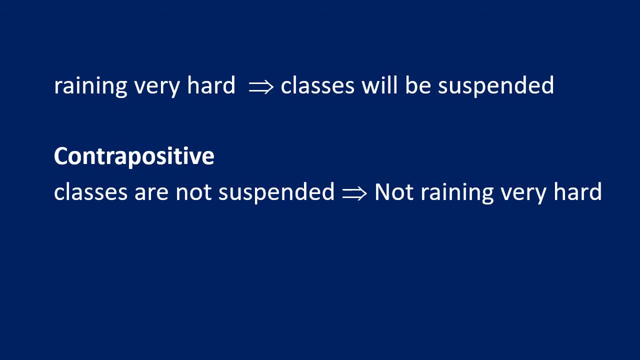 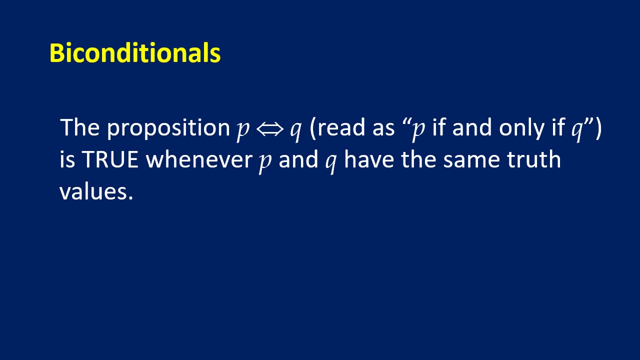 The. the new premise is the negation right, The negation of the original conclusion, And the new conclusion is the negation of the original hypothesis. Understand, OK, Let's now go to biconditionals. So we will go back to contrapositive. 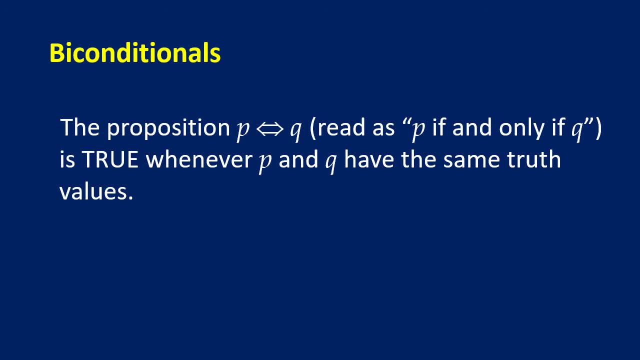 later when we talk about tautologies. OK, For now we'll go to biconditionals. What are biconditionals? It's? it's read as: P, if, and only if, Q. It is true whenever they have the same truth values. 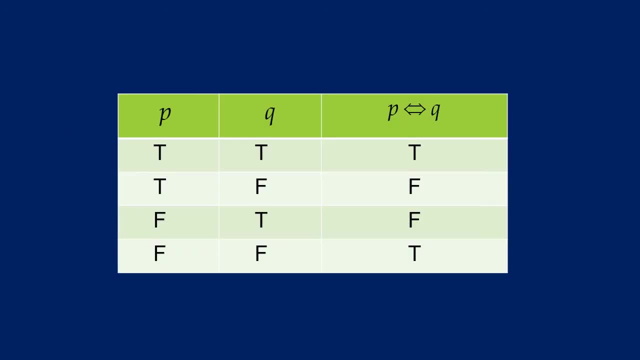 So if you look at the truth table here, it will only be true if they are. they have the same truth values. Here it's true because both P and Q are true. It is true here, because they both have the same truth value. here, F. 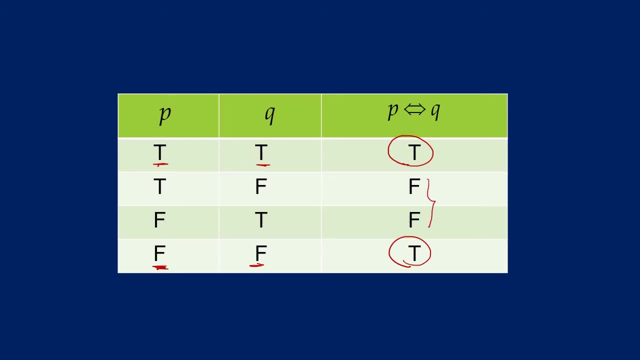 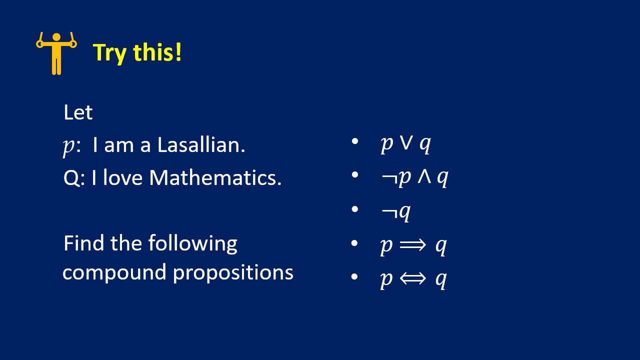 For the rest, it will be false. OK, Dapat remember that They must have the. it will be true if they have the same truth values. OK, Um, let's just um. I have sentences here. You just give me what would be the equivalent sentences. 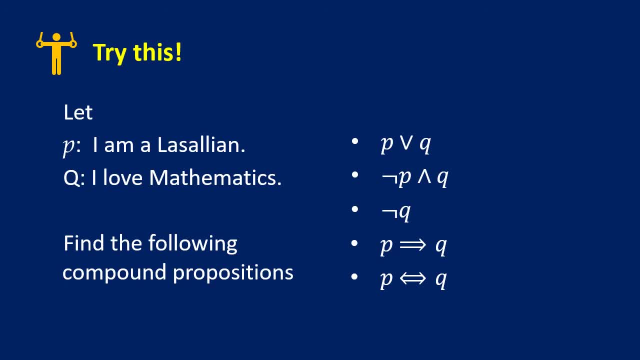 OK, so for example, this one: the statement P is I am a Lasallian. Statement Q is I love mathematics. What would be the proposition P or Q It's I am a Lasallian Or I love mathematics, correct. 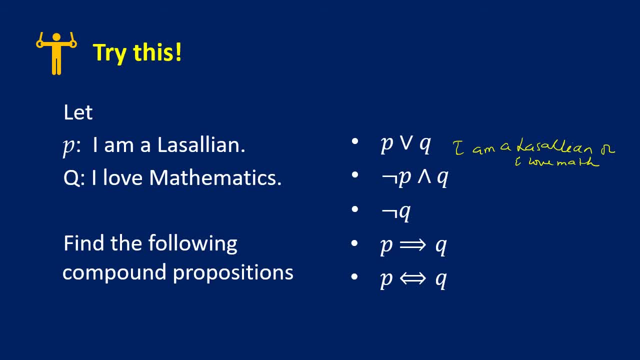 Not P and Q. Maybe I should just write it here, because I do not have space: Not P and Q. What is that? I am not a Lasallian And I love mathematics. OK, What about not Q? Of course, that statement is: I do not love. 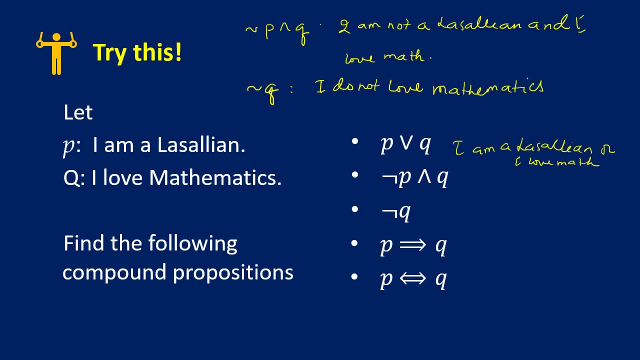 mathematics. The statement: if P, then Q is: if I am a Lasallian, then I love mathematics. I wonder if this proposition is true or false in your case. OK, And lastly, we have. let me just write it here. 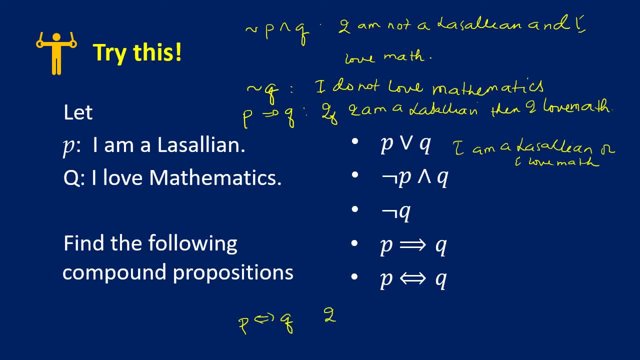 P, if and only if Q. So I am a Lasallian If and only if. I love mathematics. When I was in high school I thought the word if and only if was some sort of arte lang to give emphasis. I was already in college when I learned that it's not true, pala. 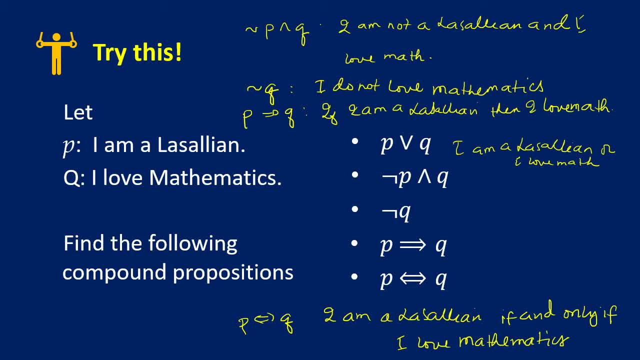 OK, so remember that whenever you have the statement if and only if, that means that if one is true, the other one must also be true. For example, if you recall this statement: in geometry and a triangle is equilateral if and only if. 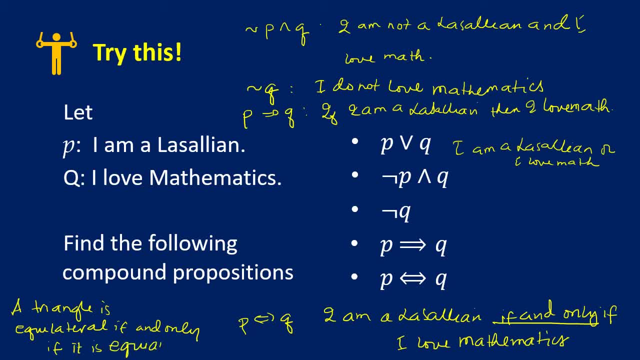 it is equilateral, Equilateral, Equiangular. So remember for a triangle, if it is equilateral, automatically it is also equiangular. So meaning to say they are the same lang, They are basically the same sentence. 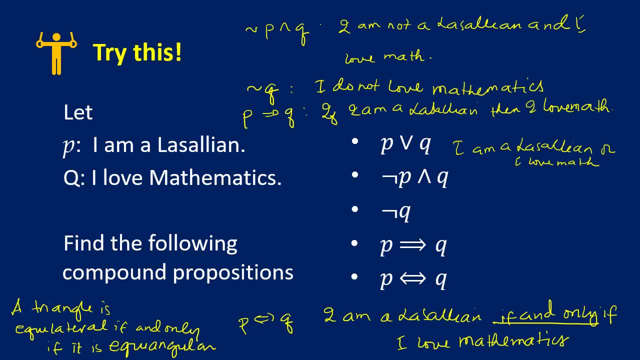 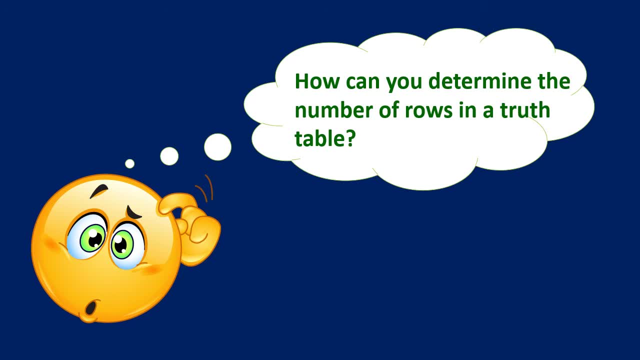 We will again. I will discuss more of that when we go to tautologies. OK, Now how can you determine so in the examples that I gave you for all of them, we just had two propositions, P and Q, and then we were combining them. 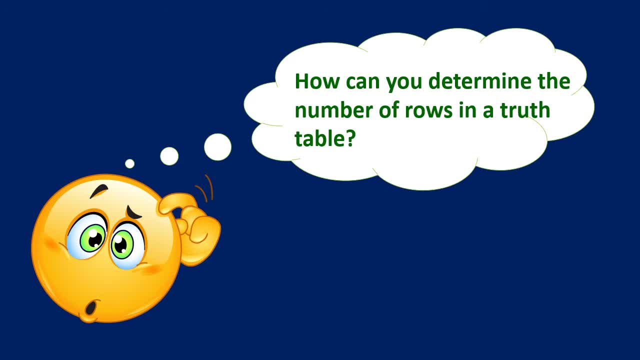 What if we have already more than two variables? How can you determine the number of rows in a truth table? Now, the answer is simple. If you just follow the the tree that I showed you, you will be able to determine the number of rows. 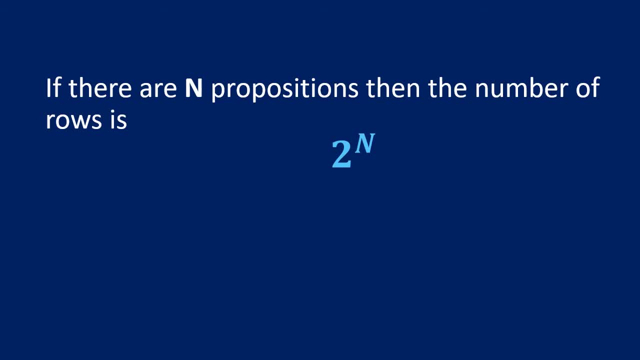 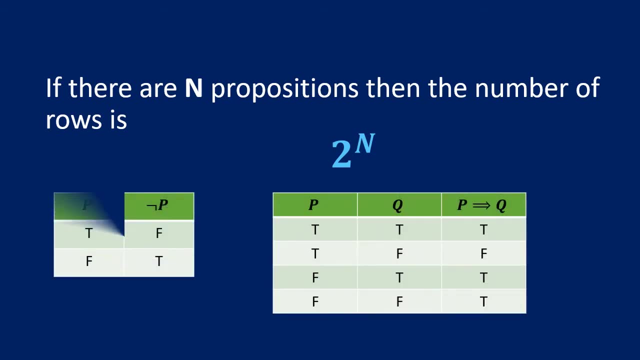 Take note that the number of rows: if you have n propositions, the number of rows would be two raised to n. For example, here you have only one proposition, right, So that's why the number of rows is two raised to one. 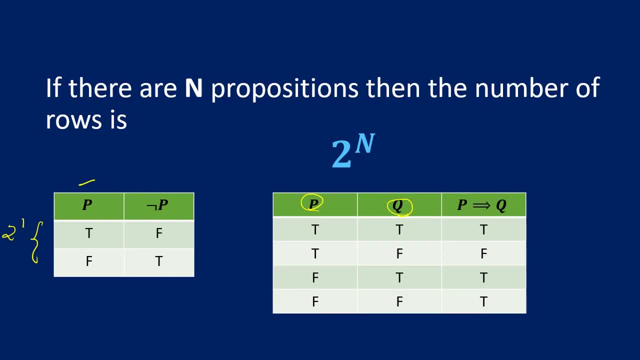 Here you have two propositions, P and Q. So that's why the number of rows is two raised to two. So meaning to say, if you have three propositions and then you are combining them using connectors or connectives, how many rows would you expect? 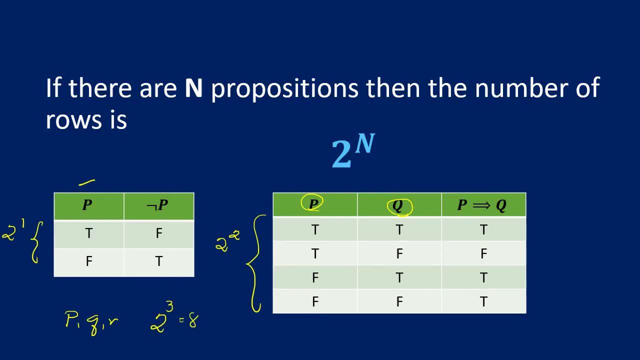 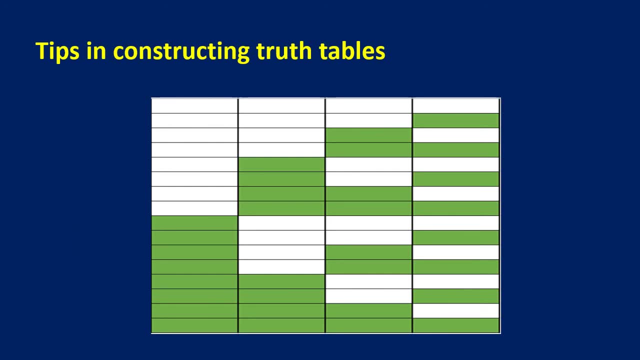 You will get two raised to three or eight rows. OK, so this is a tip in constructing the table. So what do the white and the green mean? So what this means, for example, the white, it will be true white, And then F, that would be the green. 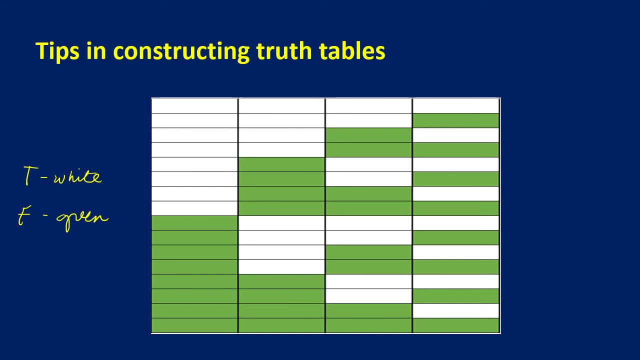 OK, so meaning to say here: if I have- In this case I have four columns, so I have P Q R S, correct? So I have four propositions. So that means, how many rows do we expect to raise to four or sixteen? 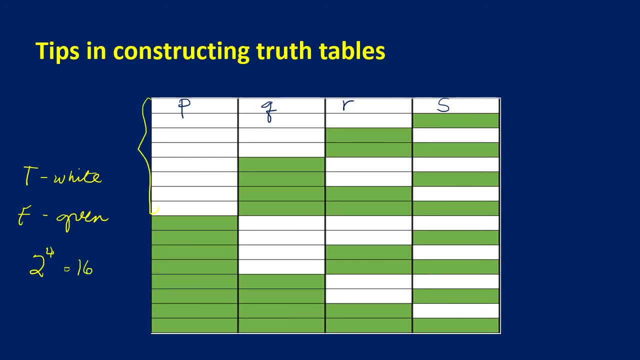 So, as you can see, here we have sixteen right, Eight here And then eight here. So what you do for the first column? you divide it into two. The first half, everything would be true, And the second half Here. for the first half, everything is true, because that's represented by white. 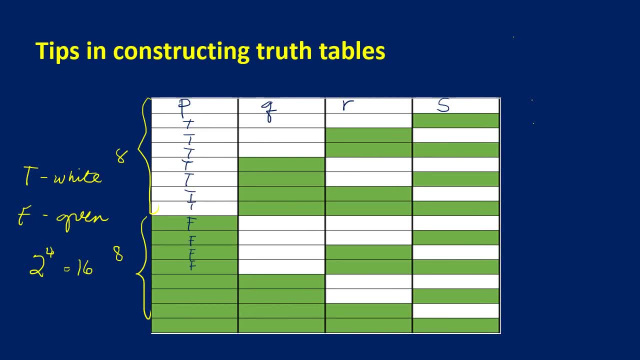 And then for the second half, everything would be false. OK, and then next ito, and then you get the half again. for this one get the half of eight. So that's why, Oops, actually this one should be part of the. 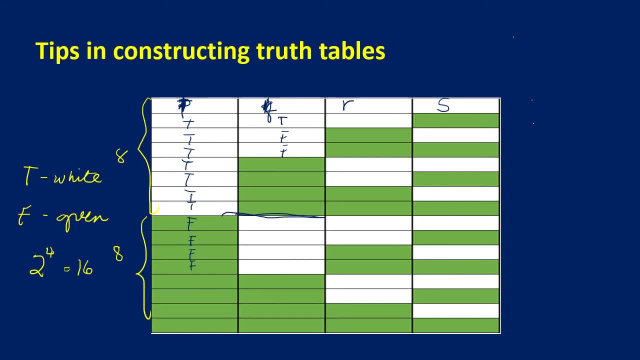 Wait, I'll just erase it. let me just Release, because that's part of the number of rows. I should write my propositions on top. So this is for P, Q, R, S, OK, And then T, right. 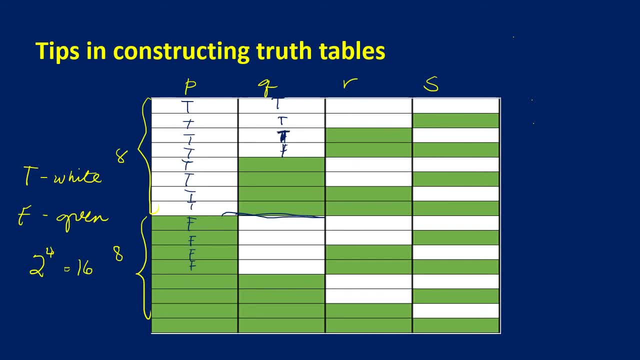 And then another half. Wait, this is true, True, true. Then green is false, And then another true again. Then repeat the process And then, like that, get half of four. So you get two first, two rows two, and so on and so forth. 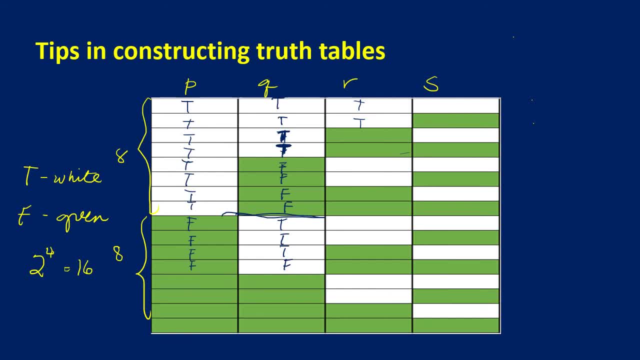 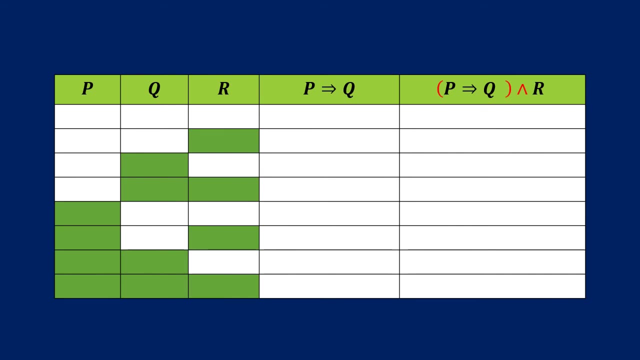 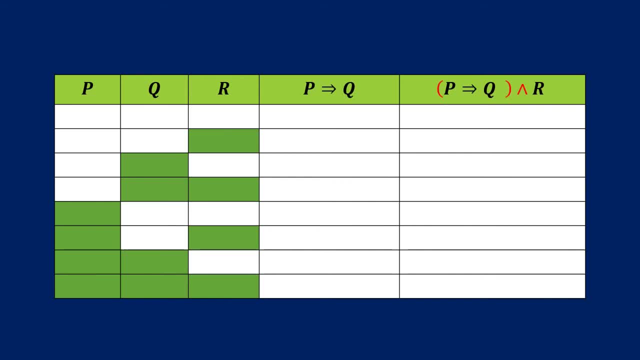 Now take note this: for this one I already gave the columns, but suppose you just have. I just gave you if construct the truth table, for if P, then Q and R, OK. So for example, you were not given the columns. 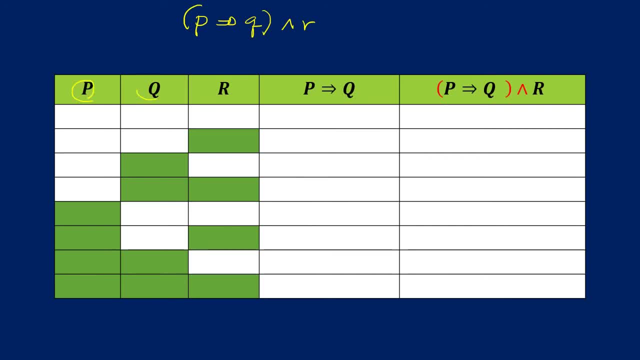 So I know that, OK, I need my. I have three letters appearing there, the propositions. So you have your columns for P, Q and R, And then what will you do You make a column for? for this one? 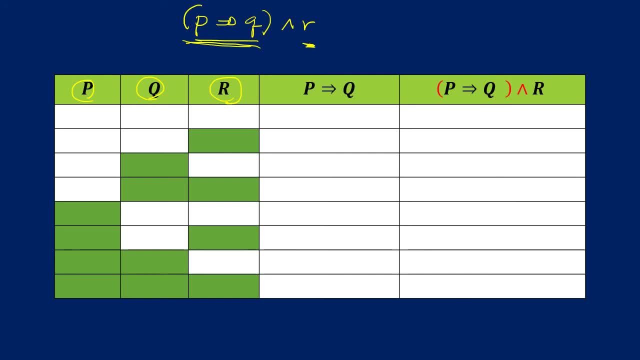 You have to because this is, you're joining these two statements, right, Correct. So that's why you have to make a column for if P, then Q And lastly, I already have a column for R And then the whole thing now can now make this column. 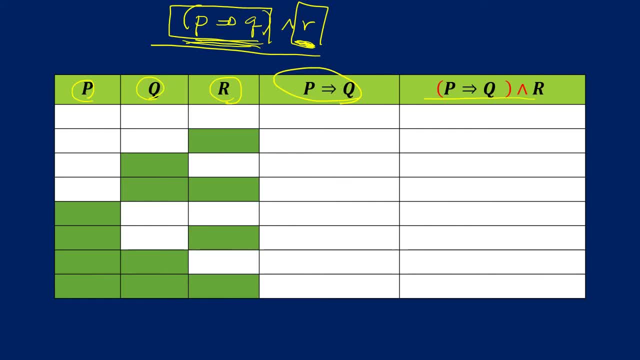 OK, so let's proceed. Let us now construct the truth table: True, true, true, false, True, true, false, false, true, false. You can also join me. no, Because of paper, you can also do it. and then, 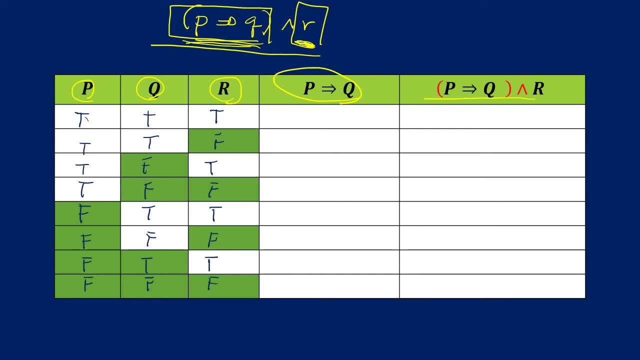 try to pause the video and then watch later. if your answers are the same as mine, OK, so first for this, for this column. if P, then Q, remember? So that means we are looking at the. what are the components? 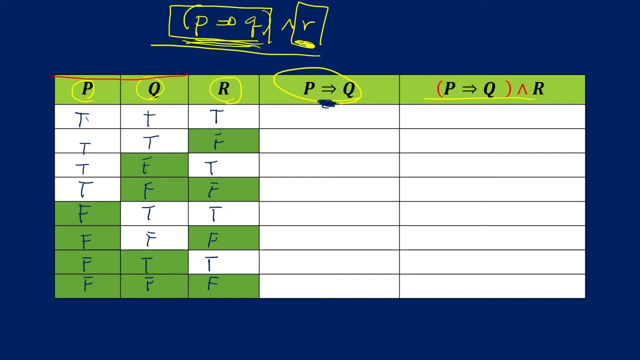 You are looking at these two columns, right? If P, then Q. Remember, it is always true, except when the premise is true but the conclusion is false, and it occurs here, Right? That's the only case wherein the premise is true but the conclusion is false. 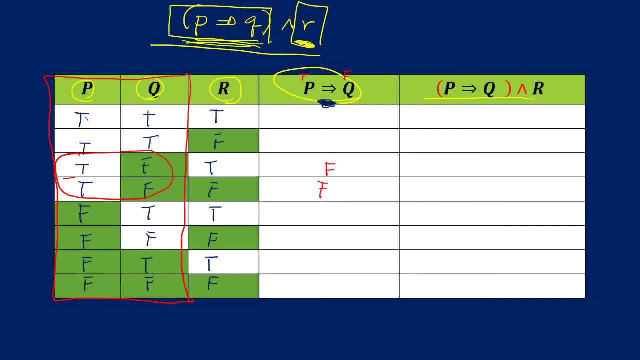 So that means it's just false here, And then for the rest it is true, OK. next for our last column. we are looking at this one. We are joining these two parts. if P, then Q and R. So that means 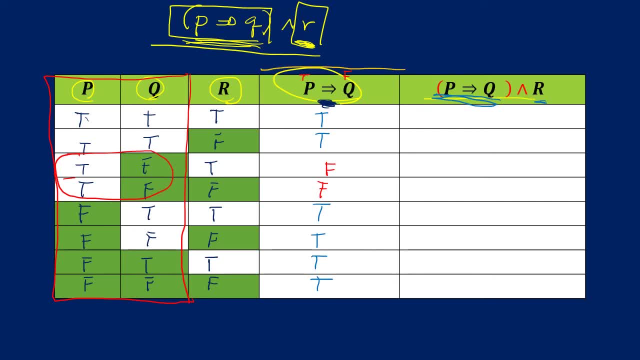 we will look at this column. This is the first component, right, And the second component is this R. so this one, Remember: for, AND it's commutative. It doesn't matter which one will come first, right, And also for, OR maybe we will talk about that later. 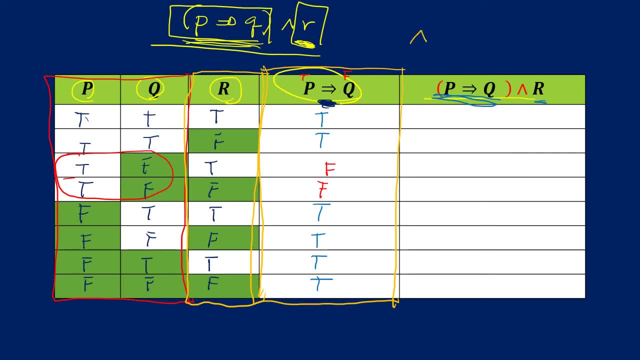 But anyway. so remember that for AND when it will be true. both are true. So when are they both true? So for the first row, they're both true Here, no, Here. Here they're both true. so this is true. 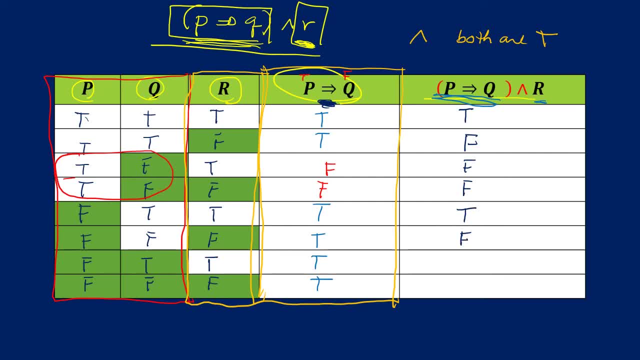 Here, one is false, one is true, So the statement is false. And then here, both of them are true. And then, lastly, you get false here. So that's how you construct the truth table of this proposition. All right, so let us now construct the truth table for. 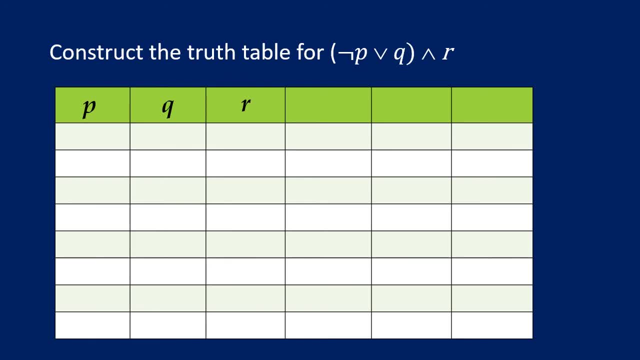 not P or Q and R. All right, what are the columns that we need for this? If we take a look at this, this is: you're joining two statements- not P or Q, and the other one is R. So that means I need a column for not P or Q. 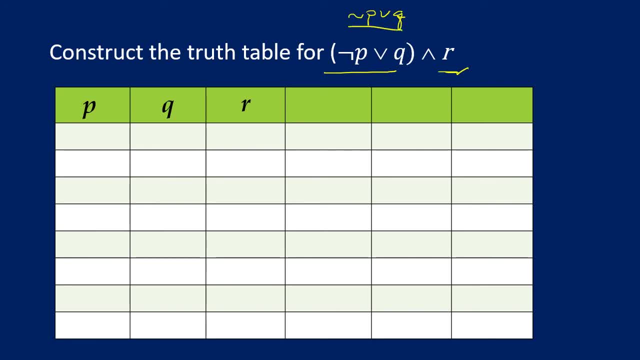 I already have a column for R. However, before I can make a column for not P or Q, I need a column for R. So I need a column for this: is you're joining not P, and then Q, So I need a column also for not P. 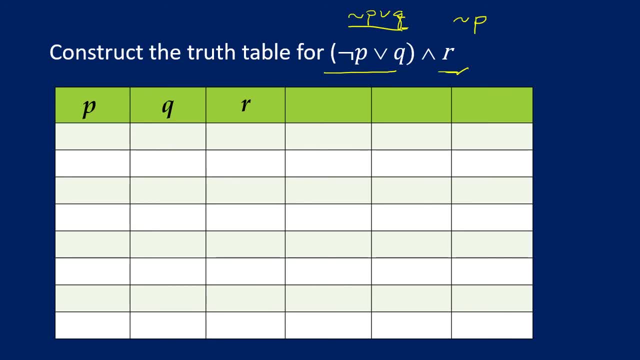 I already have Q right, So let me now write those. I need not P to get, not P or Q, And lastly, what I want is not P or Q and R. okay, So we're now ready to fill in our table. 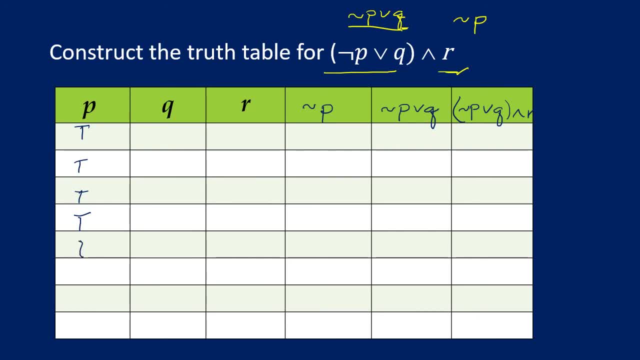 So first half is true, false, and then next half, And then true, false, alternate. Okay, for not P. we just look at the column for P, the opposite of that. So we get four false and then for true. 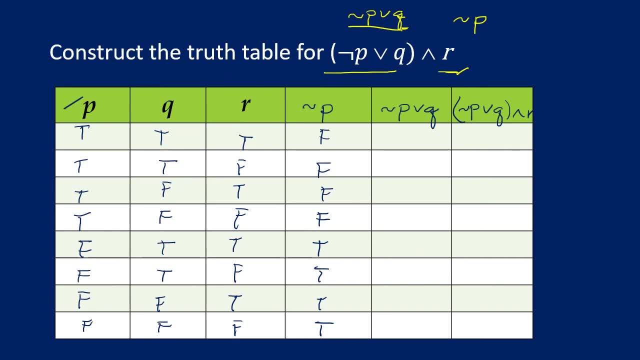 Okay, now we have not P or Q, So or so we are looking at the components this column, Not P or Q. So what is the truth? when is the statement, or again, true? We need at least one to be true. 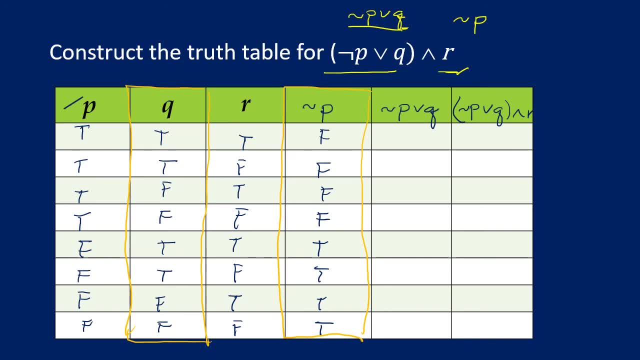 Correct. So for this one, what is it true or false? You have one true: Q is true, So this is true. And then this is true. For this one: none of them are true, right? So this is false. 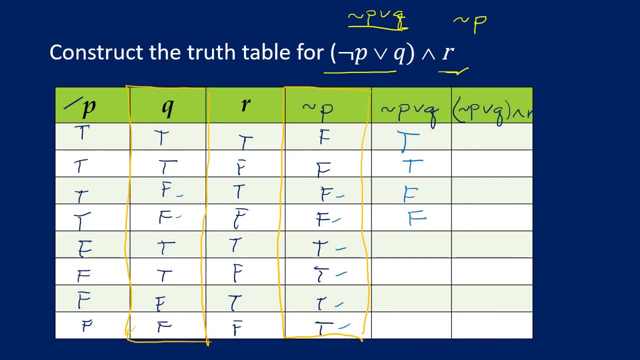 For here this is, since not P, one component is already true, So that makes the entire thing true already. And lastly, not P or Q and then R. So we will look at that. what are the components? not P or Q. 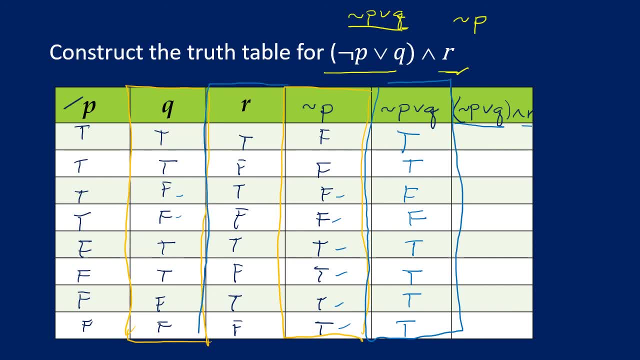 and then the state column R: Okay, so we want it. maybe I should highlight, Highlight, Highlight, Highlight, Just so that it will be easy for you to look at which two columns we are doing. Okay, So, and remember when is they are connected by, and so therefore, they must be both true. 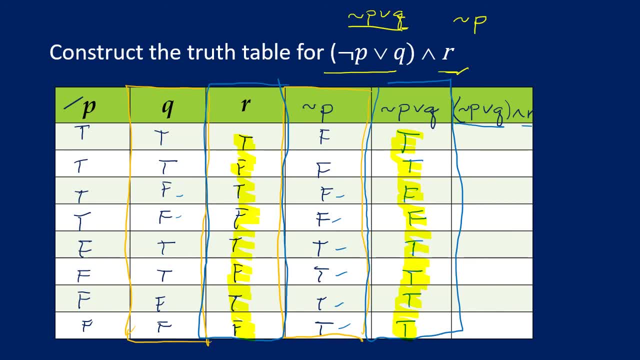 to become for the entire sentence to be true. So therefore, here for the first row. they're both true Here, false, false. none of them are true here, False here. they're both true, False here. they are both true and here. 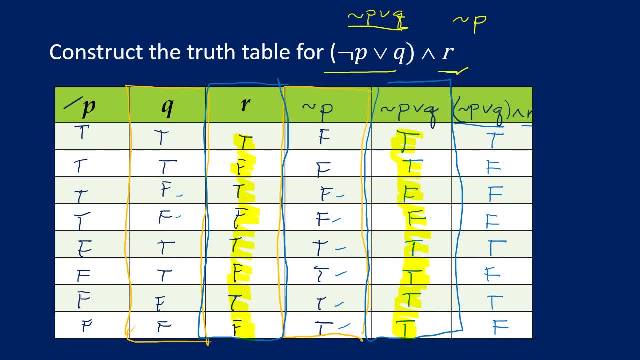 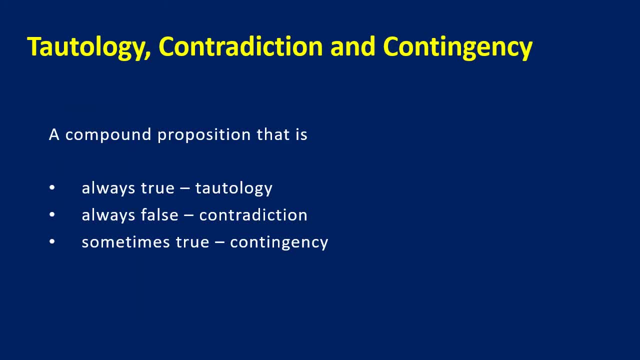 Yeah, so this is now the truth table for this proposition. Is that clear? Okay, let's now go to tautology's contradiction in contingency. A compound proposition- that is always true. It is said to be a tautology, always true. 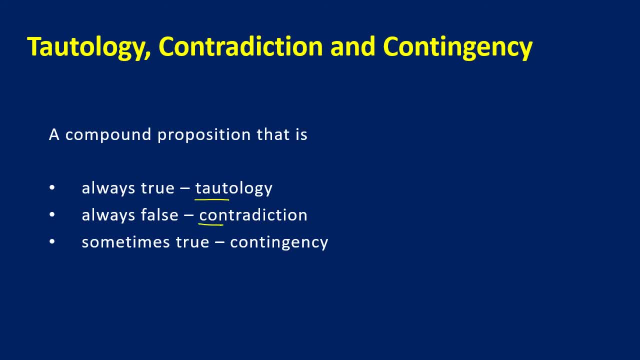 If it's always false, it's a contradiction, And if it is sometimes true or sometimes false, it's called a contingency. So, actually, the truth for the truth, for the two truth tables that we constructed a while ago. what are they? 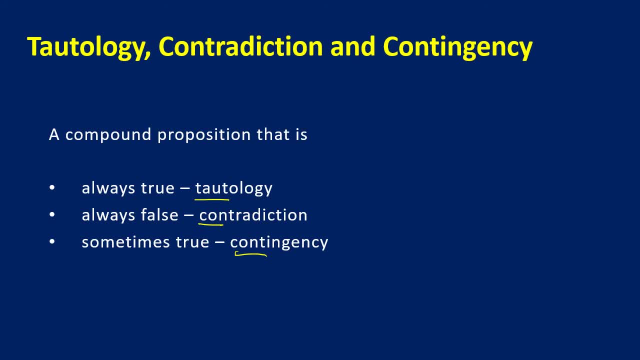 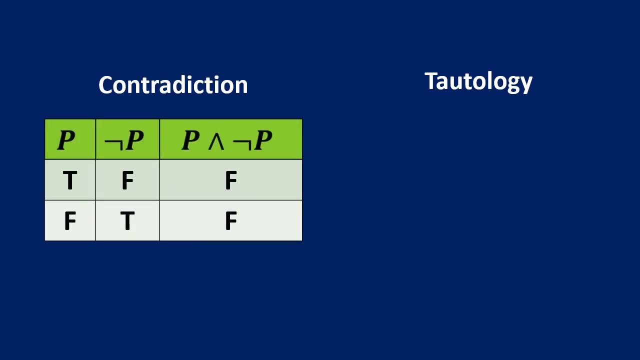 They are both contingencies right, Because we have rows wherein it is true and then we also have rows wherein it is false. So I will give you an example of a contradiction in a tautology. So this is a contradiction: The proposition P and not P is a contradiction because, as you can see, 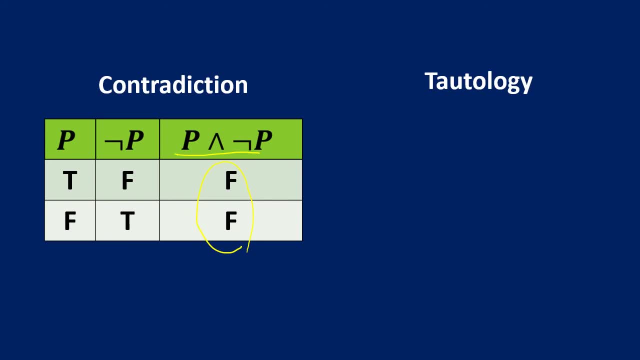 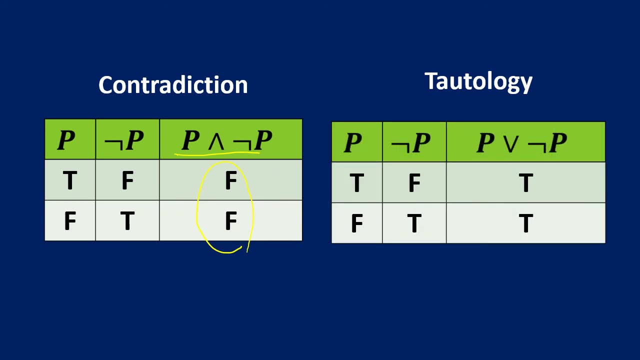 for its column the corresponding column for P and not P. it is always false. A tautology naman would be P or not P. So it's always false, Not P, correct, OK, because since always one of them would be true, right. 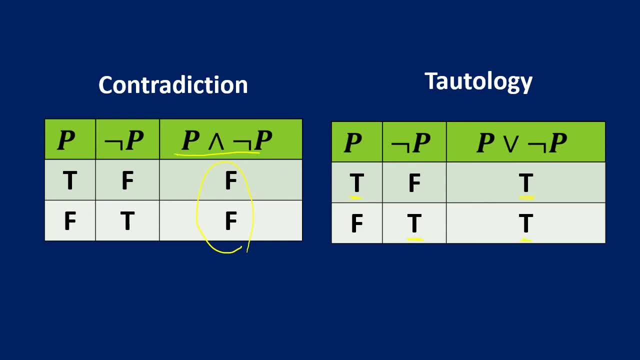 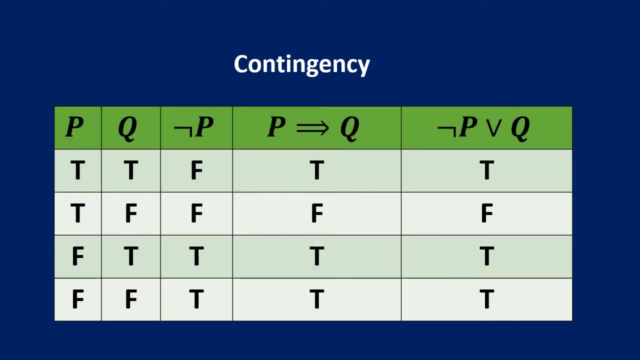 So in either case, both rows would be true. So this is an example of a tautology, because all the truth values for that particular column are true. OK, So a contingency, this one, so we have P- implies Q. that's a contingency. 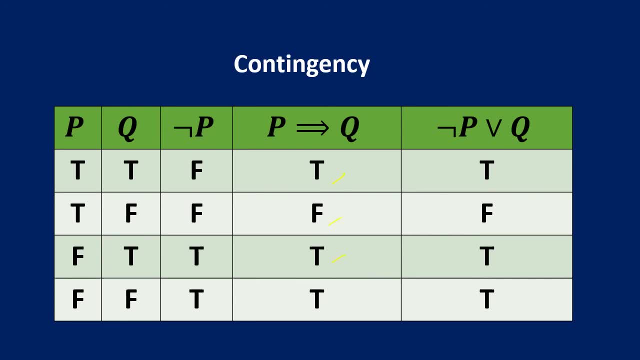 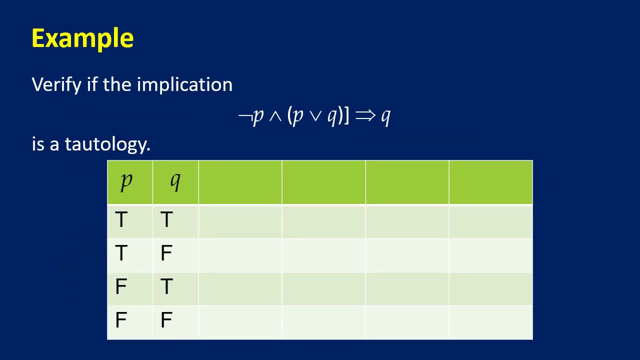 Not P or Q, because sometimes it's true, sometimes it's false, right? OK, it's a contingency, All right. So let's verify if this implication is a. if yeah, if So, we're not sure. if it is a tautology. 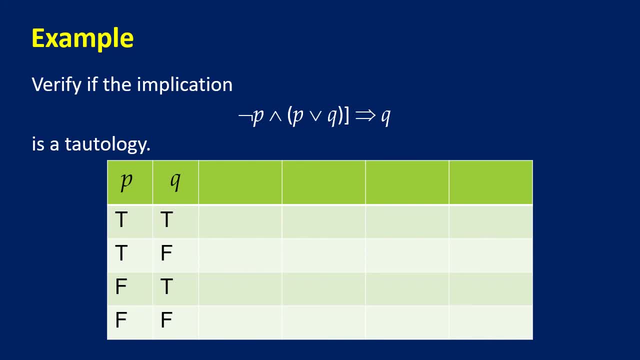 OK, so I already just have two propositions here, P or Q, So that's why we have four rows here. What are the columns that we need First? we need: OK, let's look at this right. This is actually an implication of this and this: 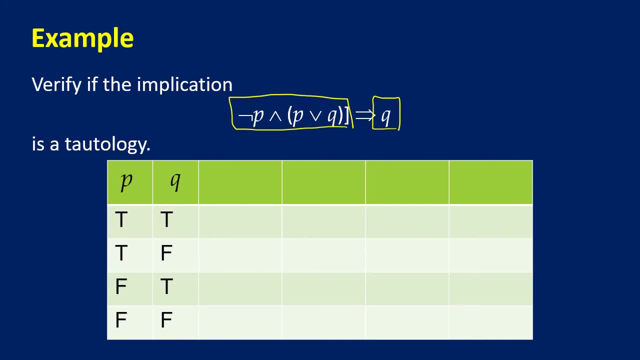 OK, so, but for this one, OK. so definitely we need a column for the last one. not P or Q implies Q, OK, but if you take a look at this one, what do we need? We need a column that's: you're joining this and this. 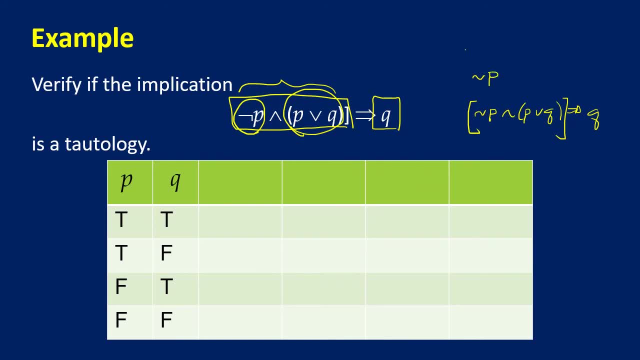 So we need a column for not P and for P or Q. Right, That's it. So we just need how many columns is that We need? I wait, by the way, we also need, of course, the not P. I forgot, of course, the not P and P or Q. 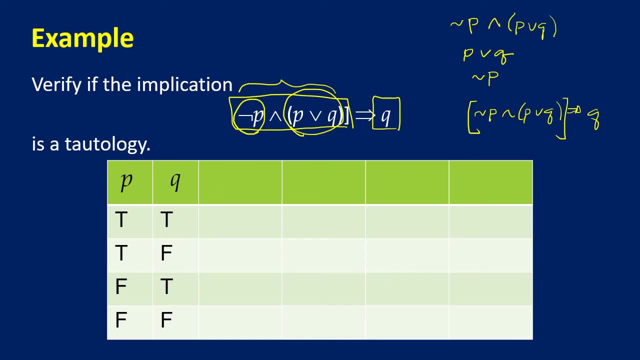 Right, So first we have not P, Not P, P or Q, Not P and P or Q, And let's just call this whole thing star. OK, the last one Star, Anyway. OK, so let's proceed. Not P, so the negation of P. 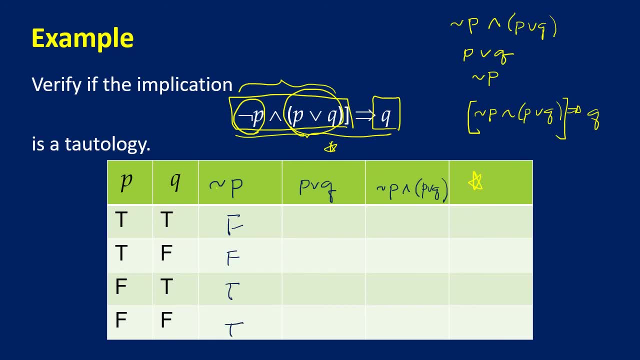 So false, false, true, true, P or Q, So we just need at least one to be true. So here it is false because none of them are is true. Next we get: we now look at this column, not P. 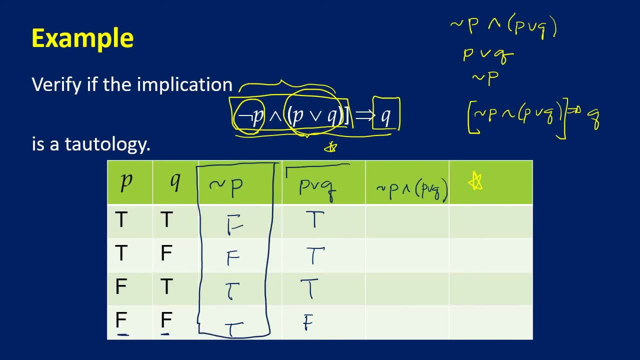 End, End For end. for it to be true, we should have both statements to be true, And it can only be ito lang yon true. For the rest, it's false. And lastly, for our star, this is the premise. 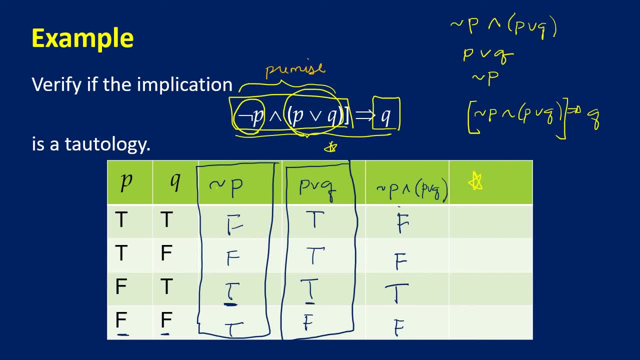 This is our premise, This thing, This is the premise And the conclusion is Q Right. When is a statement, when is an implication false? We only look at the row where it is false, when the premise is true, But the conclusion is false. 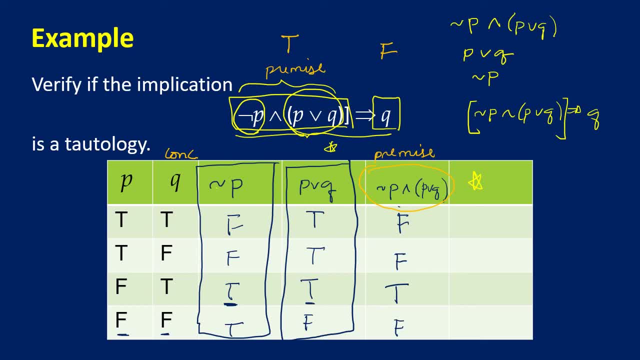 Where does this? do you have that? No, we don't have right. If you look at this, there is only one row where in it is true the premise, But the conclusion there is true. So For everything that's true. 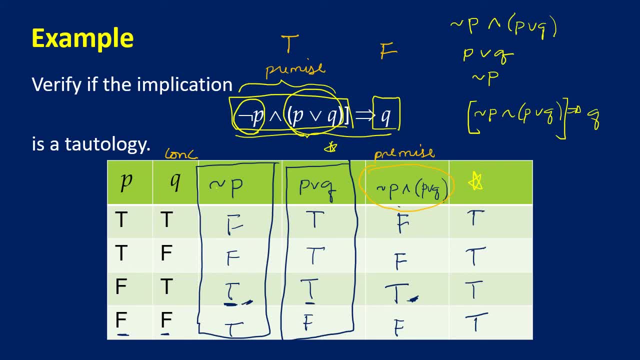 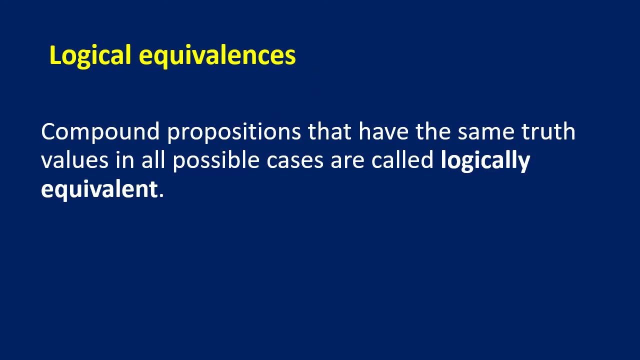 So that's why this is an example of a tautology, because the last that column this is now a tautology. All right, Next we will now go to logical equivalences. Compound propositions that have the same, that have the same truth values in all possible cases are called logically equivalent. 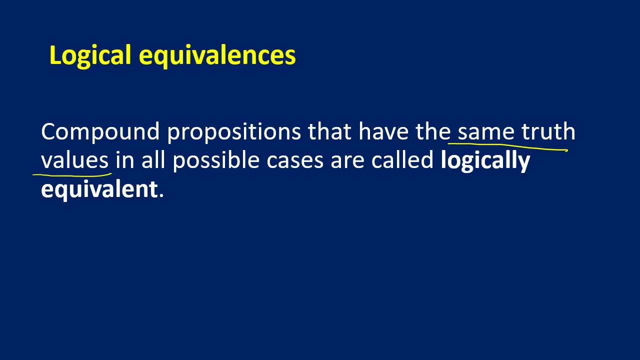 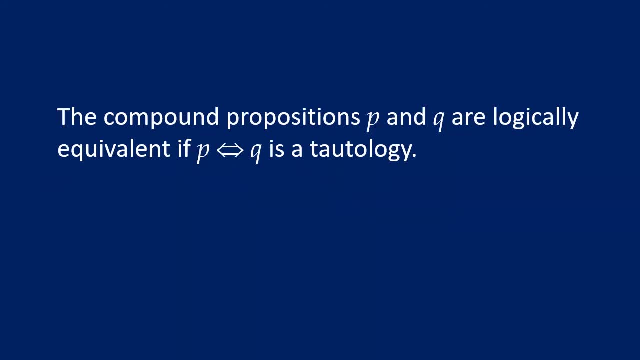 Meaning to say- take note of that- that they always have the same truth values. Whatever happens, they always have the same truth values. Now the compound propositions. another definition of logically equivalent statements is that if you form this statement, P, 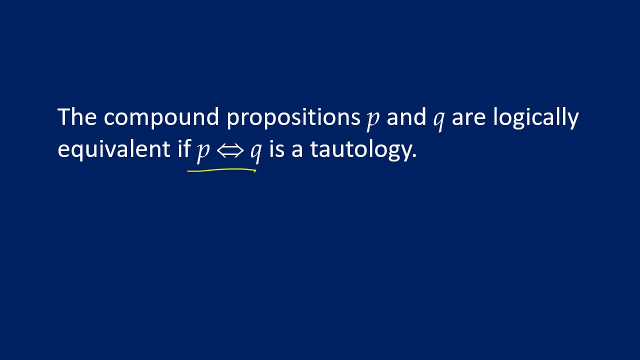 P if, and only if, Q is a tautology, OK, so what that means is that, for example, I have a proposition here, whatever star- and then another proposition. In the end, in the end, they always have the same values. 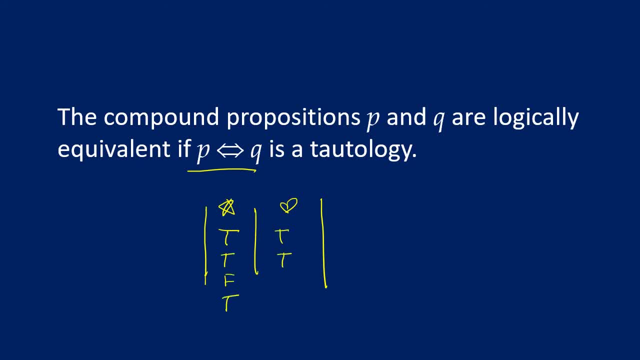 True, true, false, true, Let's. let's just say it's like that. So they have the same right, They have the same. excuse me, They have the same, They have the same truth, truth tables. Now, if I form, if that's the case, what will happen if I form the bi-conditional? 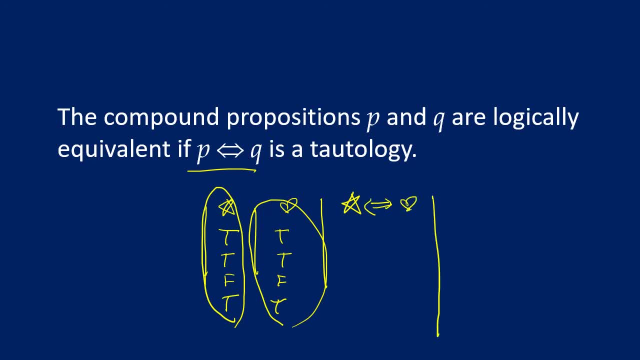 star. if, and only if, heart Remember. when is this true? the bi-conditional: It is true whenever. they have true sya kapag always, but they have the same truth values And we already know that they always have the same truth values. 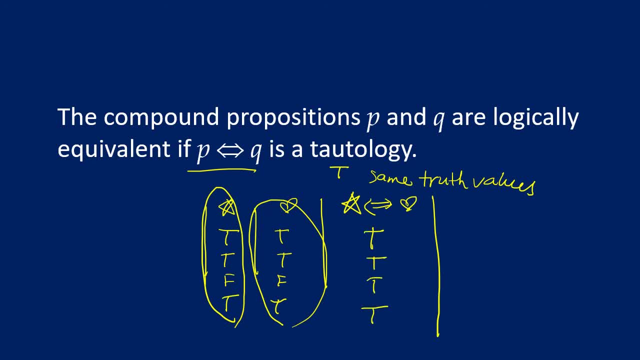 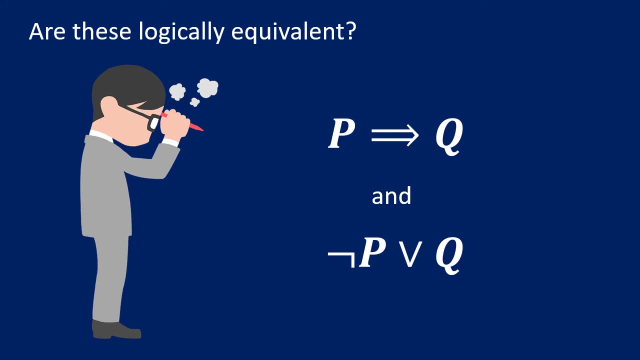 So that's why this bi-conditional is always true. So that's why, since it is always true, that statement is a tautology, OK, OK, let's look at this. one is this: are the statements: P implies Q And not P or Q? 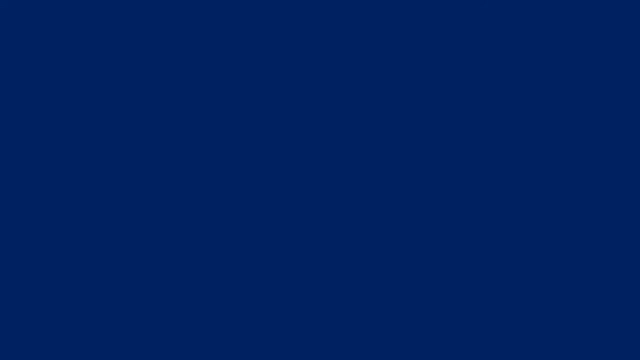 Logically equivalent. I will leave it to you as an exercise, because I already spent a lot of time doing what's this truth tables. But yes, They are logically equivalent. All right, So that's seat work. Try it for yourselves. OK, I will no longer do that. 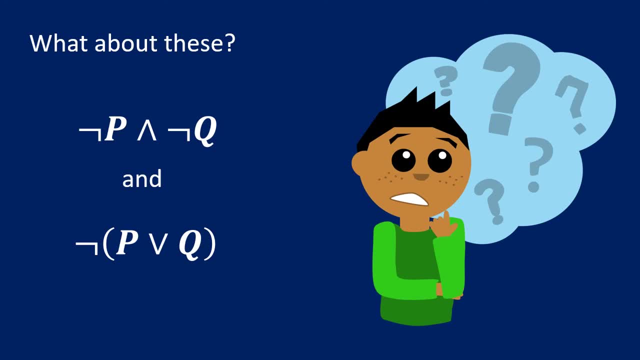 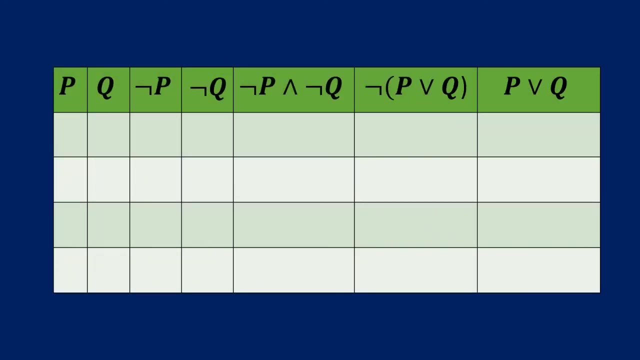 All right, What about this? not P and not Q and the statement not negation of P or Q. OK, I will do it. What are we checking again? We are checking if the statements not P or not Q is logically equivalent with the. 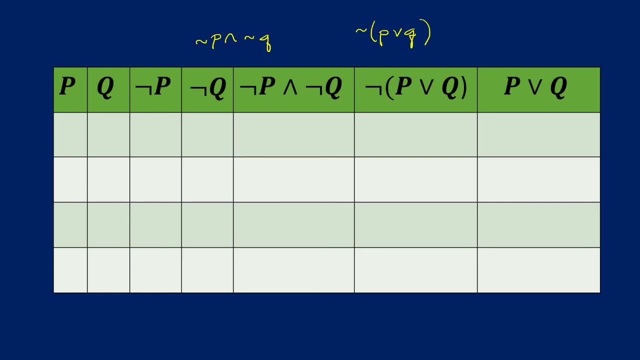 negation of P or Q. OK, so true, true, false, false, Not P, Not Q, Not P, Not Q, P and not Q. So I'm looking at this: two columns So and when. it will be true if both of them are true. 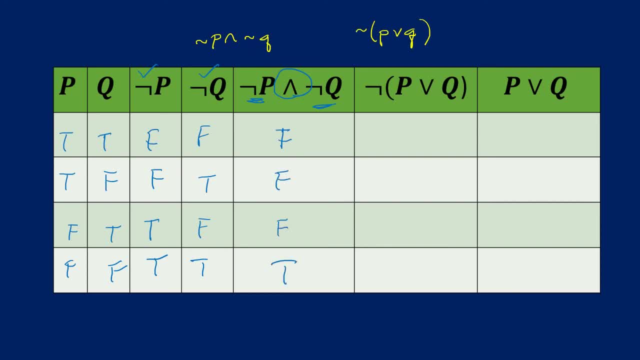 False, false, false, true. OK for this one, not P. we need this first right. P or Q. For P or Q, when is it true? We need at least one. So I'm looking at this column. 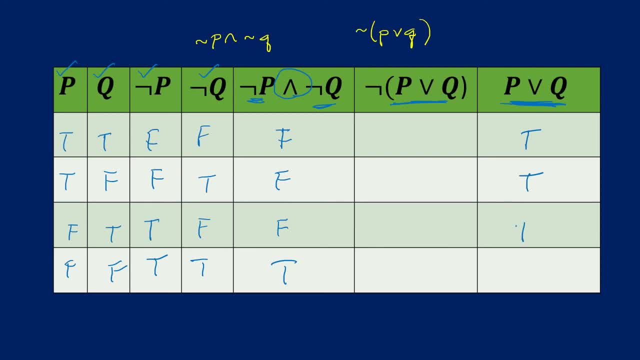 We need one of them to be true And lastly, this one. So we have the negation of this column: False, false, false, true. See, if you look at this columns over here, they are the same Same. 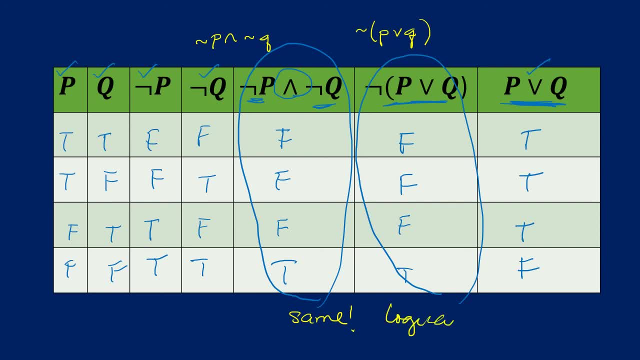 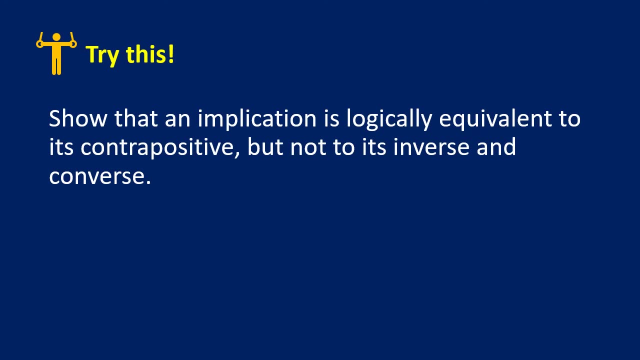 So therefore they are logically equivalent. OK, Now take note. show that an implication is logically equivalent to its contrapositive, but not to its inverse and converse. Again, I already spent a lot of time in constructing truth tables, So I will leave the truth tables to you. 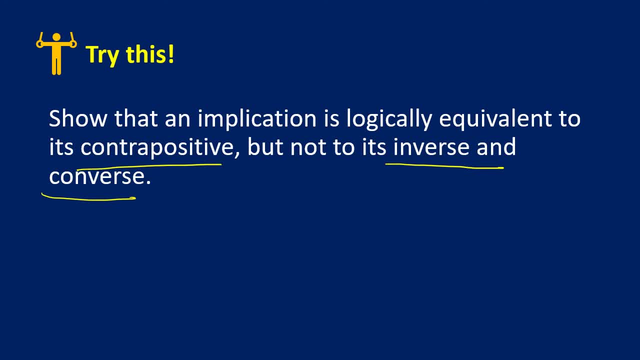 But just to show you In sentence form, sort of just to give you an example, to show you the logical equivalence of a statement and its contrapositive is this, For example: if, if I am, if I am, my favorite is Duterte. 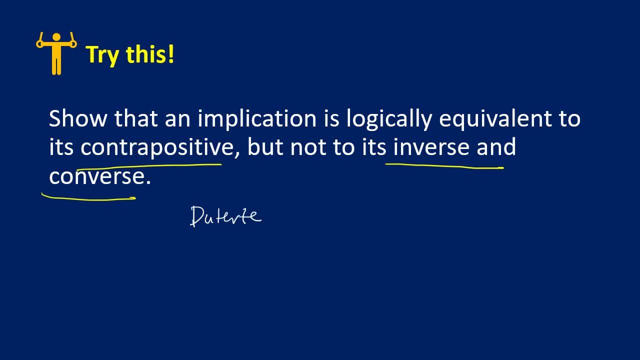 Well, I just can't think of any example right now. If I am Duterte, then I am a Filipino. OK, this is my sentence. OK, let's form its inverse, It's converse And it's contrapositive. OK, 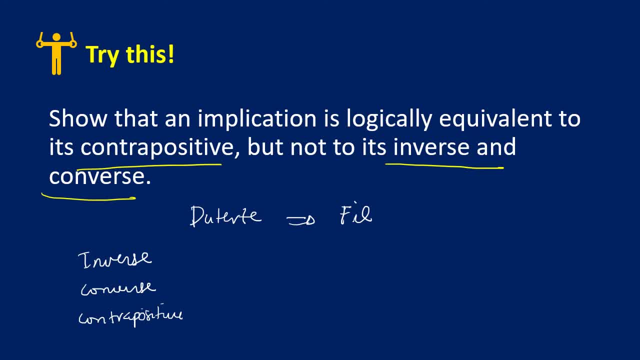 What is the inverse? How do you form the inverse? You just form the. you just negate both hypothesis and conclusion. If I am not Duterte, then I am not a Filipino. The converse: you just switch the premise and the conclusion: If I am a Filipino, then I am Duterte. 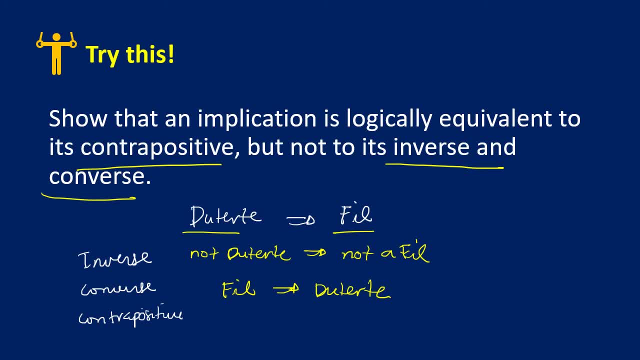 What is the contrapositive? You negate the conclusion I am not a Filipino and negate the premise Not Duterte. OK, let's look at the truth values. Let's just look at the original statement. If I am Duterte, then I am a Filipino. 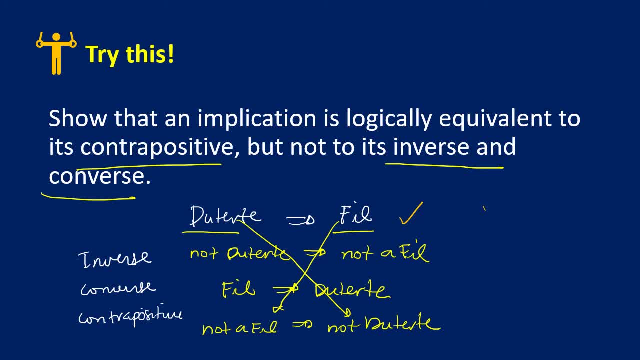 Is this statement true or false? Of course this is true. If you are Duterte, you are, you must be a Filipino. right Now, let's look at the inverse: If I am not Duterte, then I am not a Filipino. 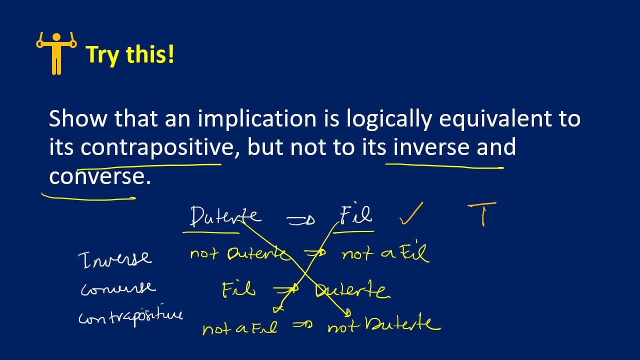 Is that statement true or false? That statement is false, right, Because we are all not Duterte, but we are all Filipinos, correct? Next converse: If I am a Filipino, then I am Duterte. Definitely false, because we are all Filipinos, but we are not Duterte. 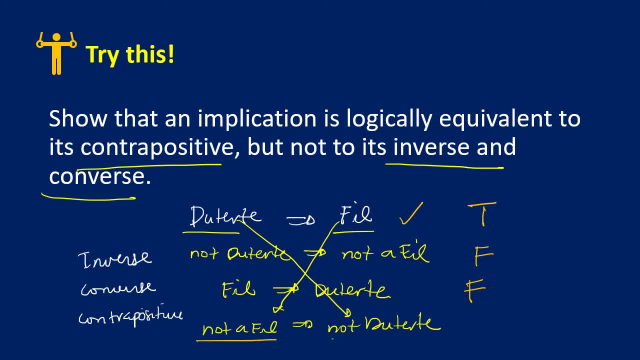 But if you look at this, if I am not a Filipino, then I cannot be Duterte, Right, It's true. So, as you can see, these two statements, they have the same truth values because they are logically equivalent. So remember when you say that two statements are logically equivalent. 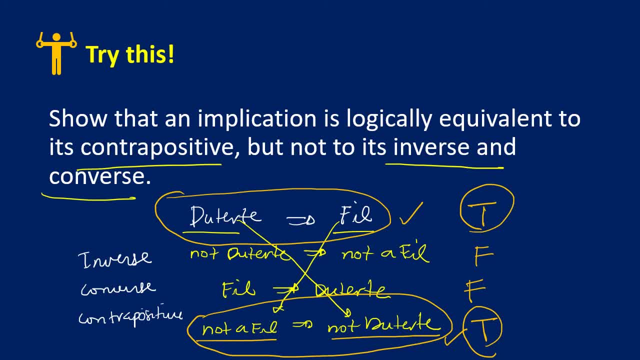 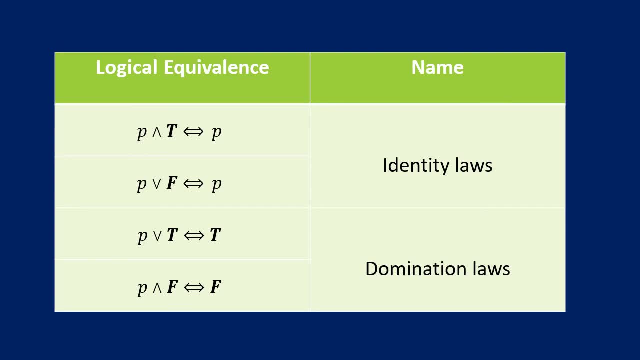 they're just the same. They're basically the same sentence. You just replaced it. OK, So let's look at these logical, logical equivalents. So we have this loss. So what is this saying? T here stands for a tautology. 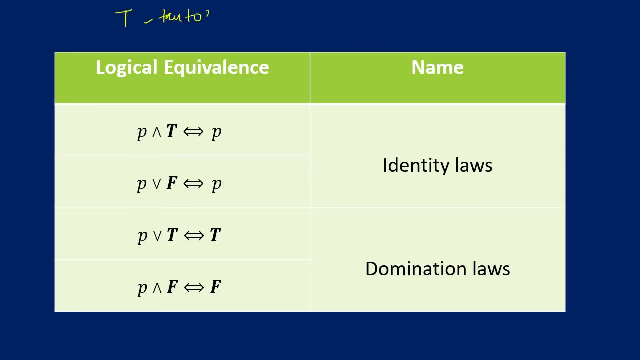 T here stands for a tautology and F stands for a contradiction. That's why he said F, because we know that for a contradiction it is always false And for a tautology it's always false, It is always true. 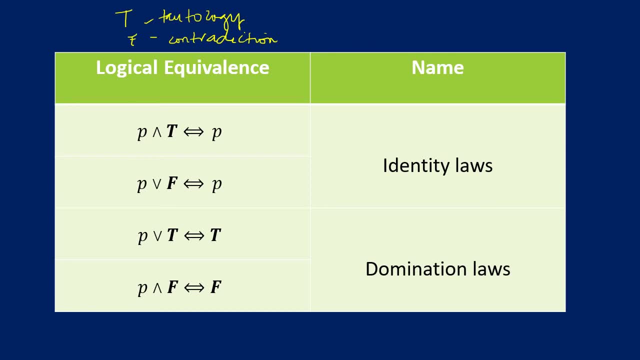 So identity loss. what is this saying? If you have a proposition, you combine it with a tautology, P, and a tautology is equivalent to P, to the proposition itself. Again, I will leave the construction of tables to show you that. 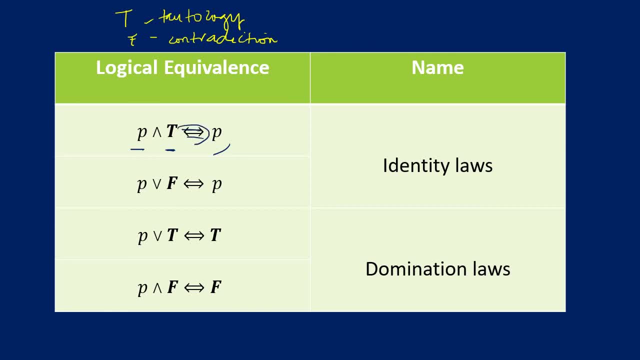 what we mean by this. actually, this symbol also. it's saying that, right, This is saying that P and T is the same, is logically equivalent to P. OK, So what we read here: they are just the same, are logically equivalent. 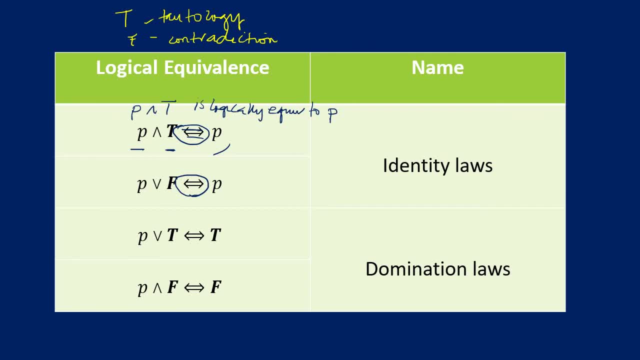 So remember, if you, if you do P and T, that's the same as P. if you join using OR, if you join a contradiction using OR with a proposition, you get the same, And that's why it's called the identity loss. 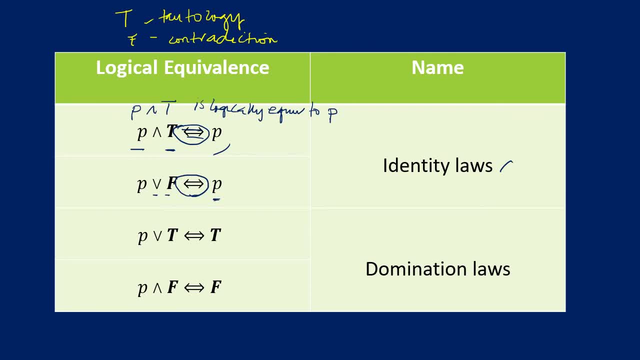 But for the domination loss, P or T is equivalent to T or a tautology. It's always true. And then P and F, it's always a tautology. So, meaning to say a tautology, you combine it with AND. 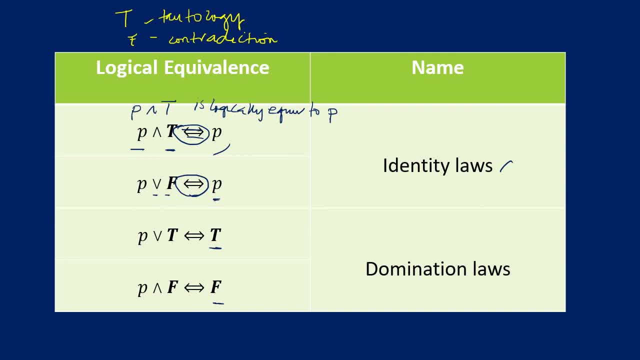 from a proposition you get the entire thing is a- I mean- contradiction. If you have a contradiction, you join it. If you have a contradiction, you join it with another proposition using- AND it's the same lang as the contradiction. 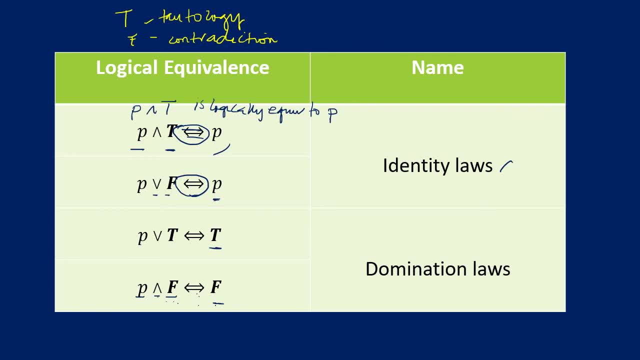 It is again a contradiction, parang ganon. Just to show you. maybe I'll just show one example. For instance, I have P. this one. I want to show that P or F is the same as P. We need the. 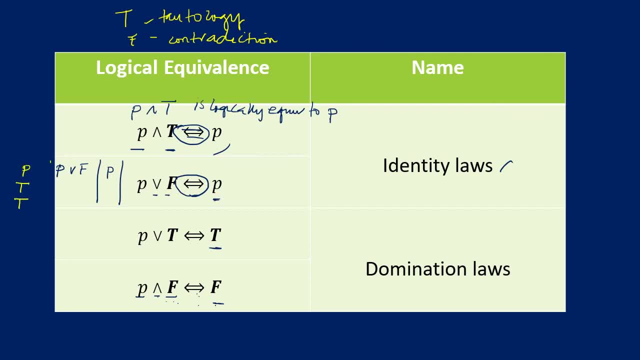 truth table for P. So T, T, correct P and F. I'm sorry, F is always false, correct, So OR? so this one We have, this is true. This one is false. So, as you can see, this is the same as. 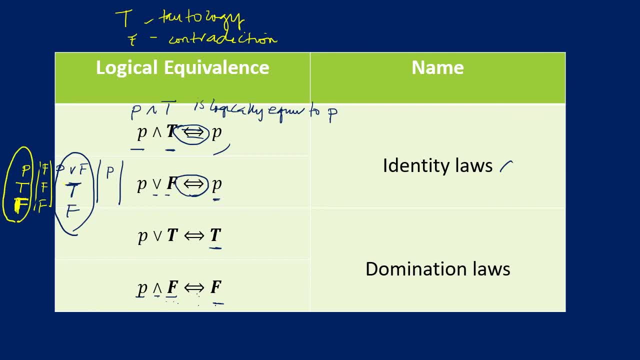 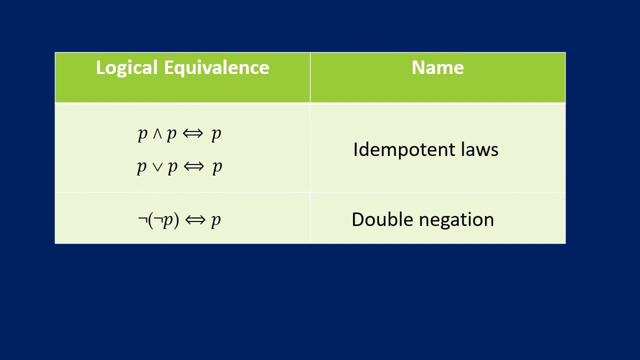 as this one Correct, OK, and then you can try the others. Next we have the idempotent laws. So if you have, if you have a proposition, and again the same proposition, that's the same lang as P, and so on. 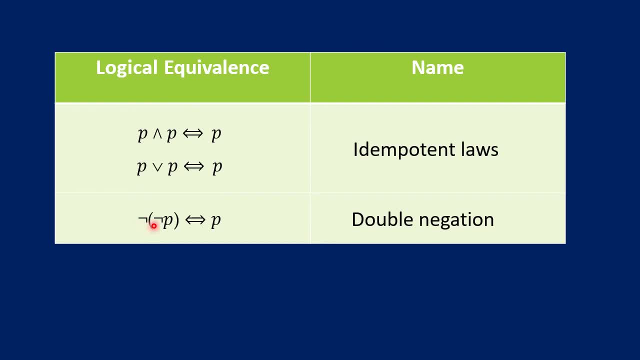 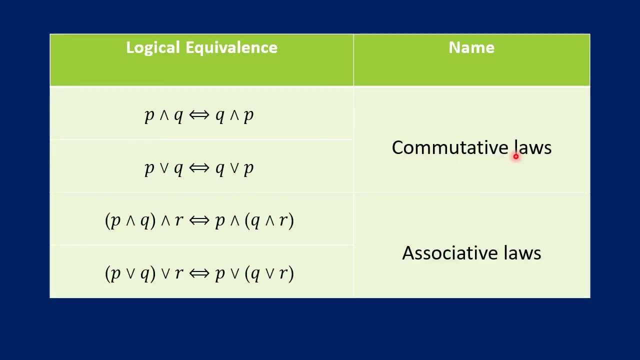 And then double negation. the negation of a negation is just equal to the original proposition itself. So it's like negative of negative of a number, It's just the number itself. Next, commutative laws. This is what I was telling you a while ago. 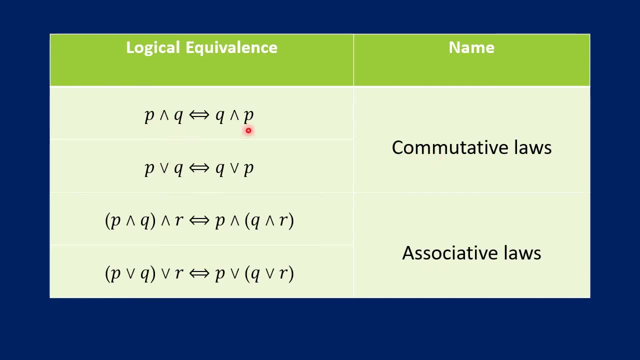 commutative laws, that if you have AND AND OR, it's just the same. If you invert them, right the ordering, the order does not matter. OK. and then for the associative laws. So it's like. it's like addition and multiplication also. 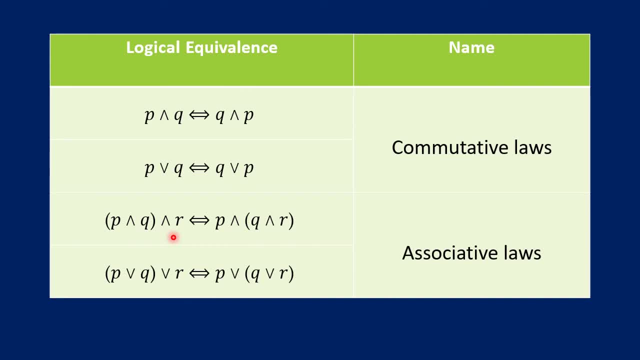 So meaning to say: if all of them- see, all of them are- AND That means the, the parenthesis- it does no longer matter. So it's like, for instance, you have P plus Q. Maybe I should not use P, because I want. 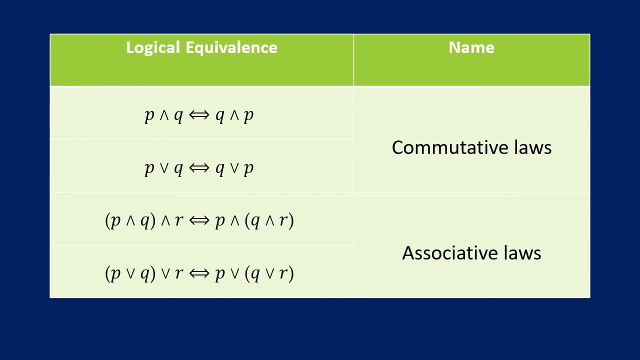 to show you that I'm looking at numbers, Let's change that We have, if A plus B plus C, this is the same, So that you can see the similarities with real numbers. A plus B plus C, right, The associative law also, right. 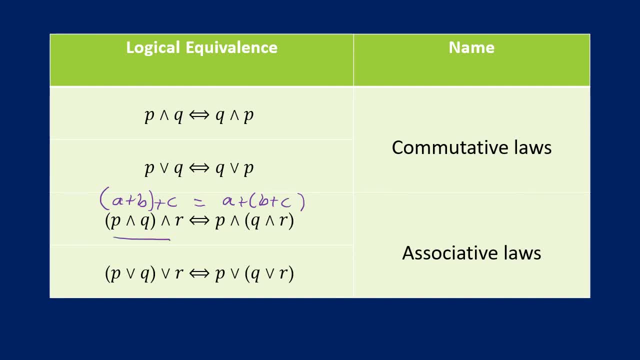 So again, what this is saying is that if all of them are the same, the parenthesis does not really matter. So here, if all of them are OR, then you no longer need the parenthesis. So that's why you can just write it as P or Q or R. 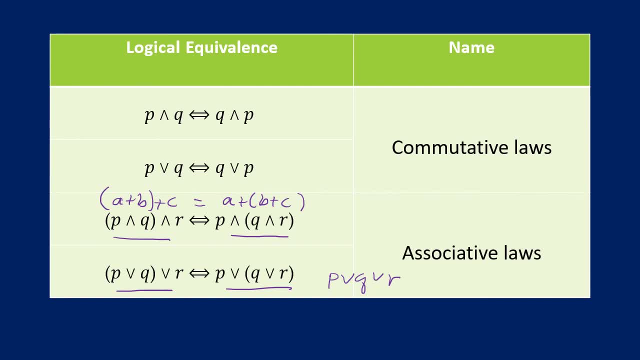 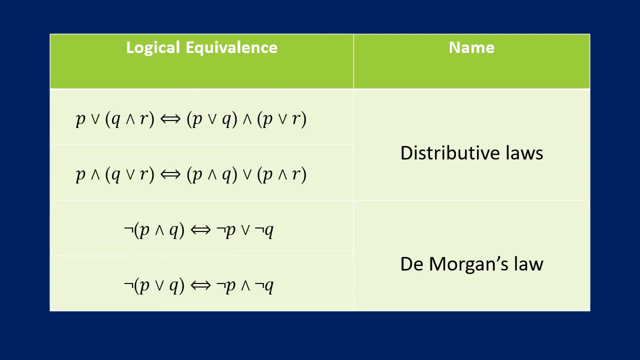 There will be no confusion because regardless of where you start, you still get the same answer. OK, next distributive law. So what's happening with distributive law? So it's like multiplication outside and then addition. So what happens if you have A times B plus C? 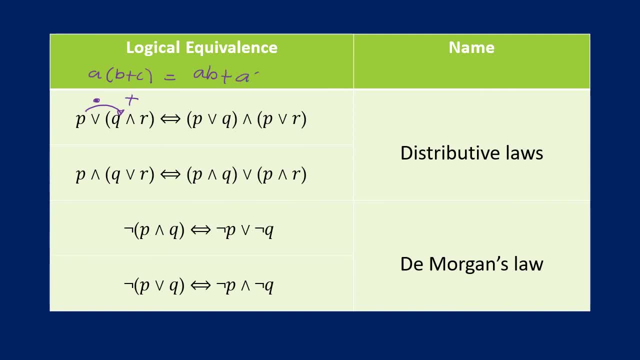 If these are real numbers, you have AB plus AC. So similarly the operation outside: OK, So that becomes like your multiplication P or Q, and then this is your right, And then distribute it here, P or R. same thing also for this one. 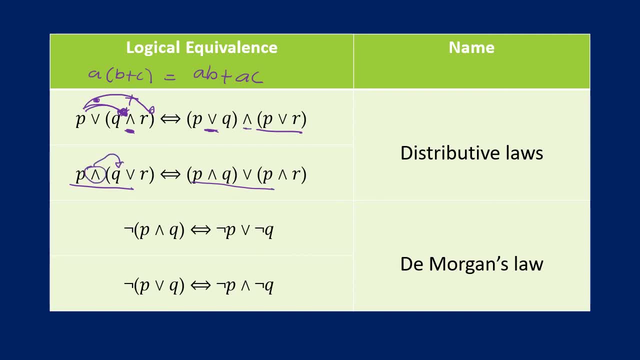 So here the N gets distributed. So that's why you have P and Q, You have P and R, And then the operation inside the parenthesis will be the operation here, The Morgans- though actually we had this one kanina, We had this right. 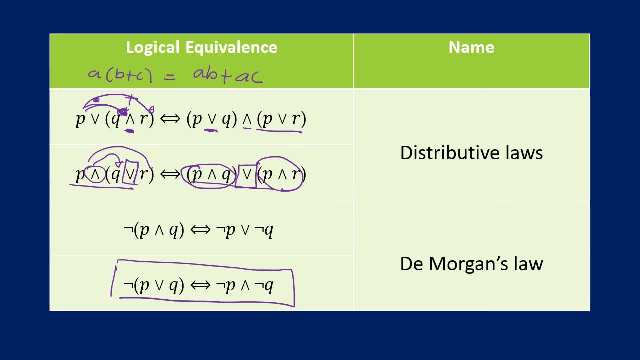 We showed that these two statements are logically equivalent Because we saw that, yeah, OK, they are the same. So what? what does the? what does the? what does the? Morgans law says. So what it means is that to form the negation of an end statement. 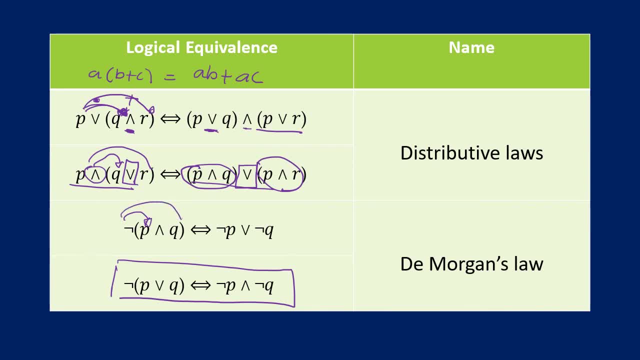 you simply distribute the negation, But don't forget to switch This one switch. If it's end, it becomes OR. So, similarly, here you negate And then the operation inside you switch, OK, OK, let's look at this example. 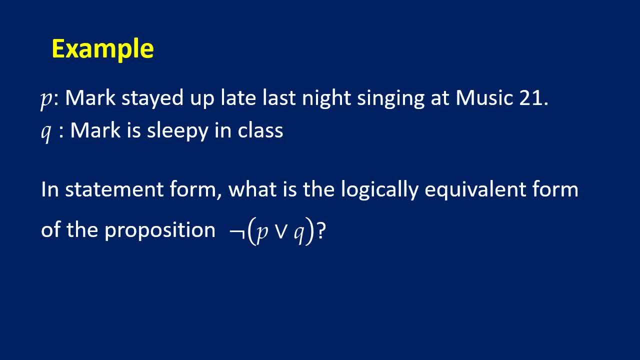 The statement P is: Mark stayed up late last night singing at Music 21.. Statement Q: Mark is sleepy in class. In statement form, what is the logically equivalent form of the proposition? Negation of P or Q. Remember that in in the English language we cannot say: it is not the case that Mark stayed up late, late late last night singing at Music 21, or Mark is sleepy in class. 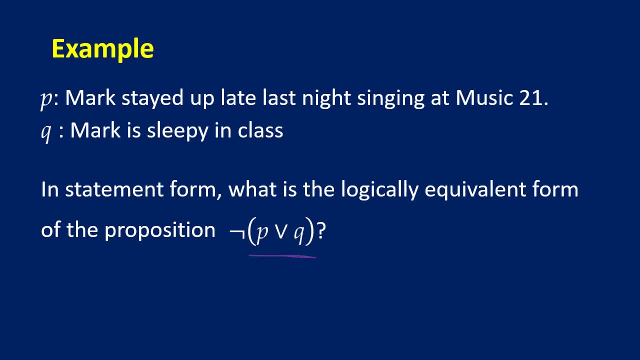 Right, Because in the English language there's no way we can. we can express the parenthesis correct, So that's why we need to express this one without the parenthesis And using the Morgan's law. what is that? That is simply not P, or it becomes end, not Q.